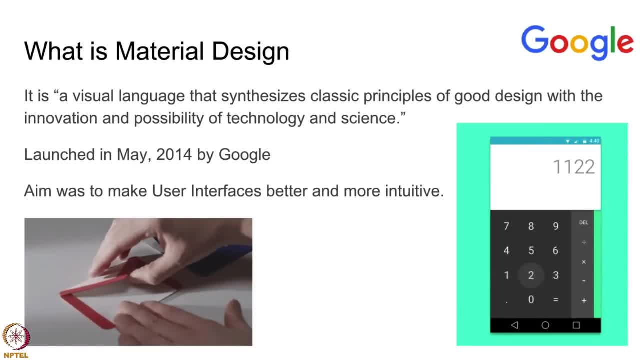 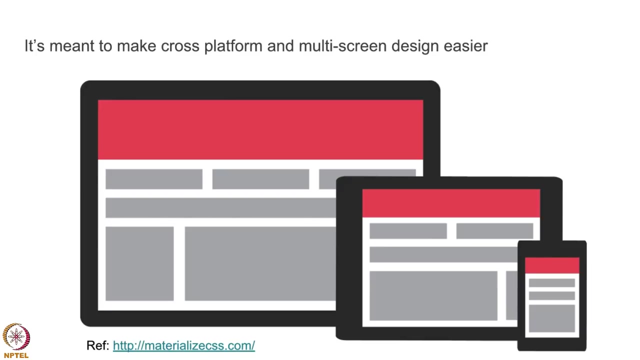 They wanted the design to be more intuitive. They wanted the design to be more intuitive. Material design is meant, toadst française, the cross-platform and multiscreen design easier so that users feel at home with the design of the system, no matter which device kids are using. 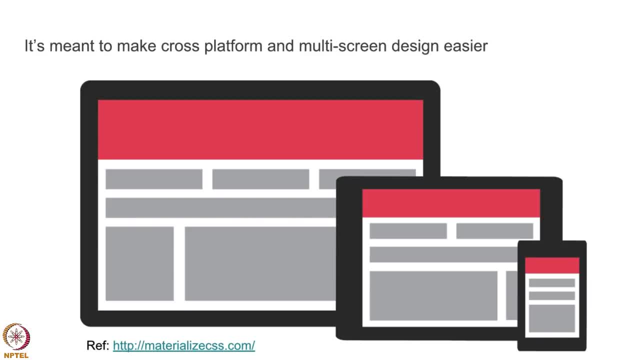 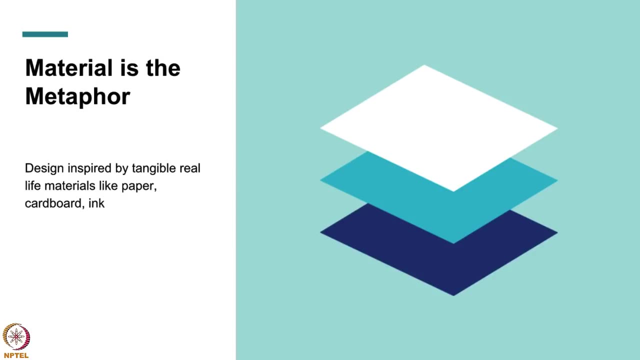 device they use it on. for example, i should be able to locate the features and functionalities of gmail, no matter which device i'm using it from, be it my ipad, my phone or my laptop. now we'll talk about the basic principles of material design. the first one is material. 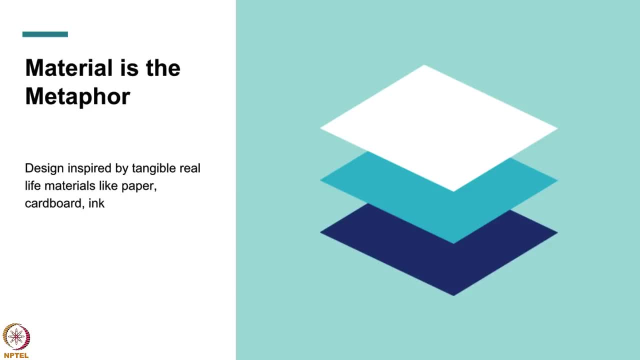 material is the metaphor. the goal is to make the design inspired by tangible real life materials like paper, cardboard or ring. tangible is something that we can touch and interact with. the feeling on the screen should be such that it should feel as if you're interacting with real 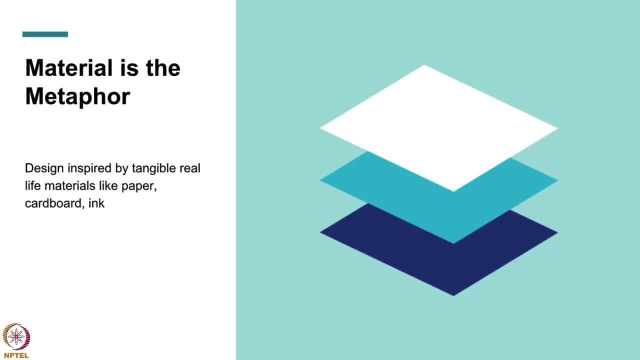 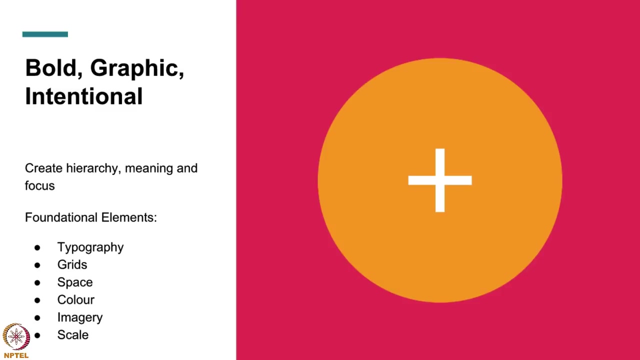 life elements. the surfaces and edges are designed in such a way that it makes us feel close to reality. light, surface and movements play a key role in defining this. realistic lighting shows seams, divide spaces and indicates moving parts, making it seem lifelike you. the next one is bold, graphic and intentional design. bold design creates hierarchy meaning. 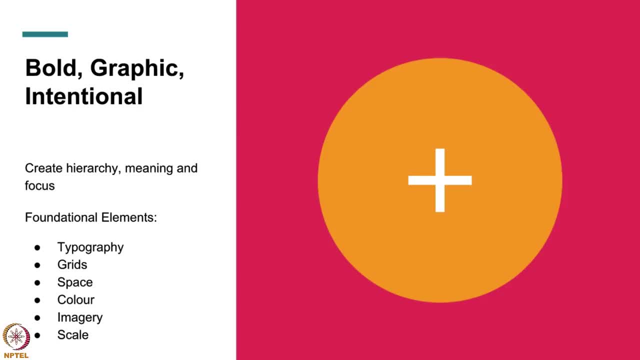 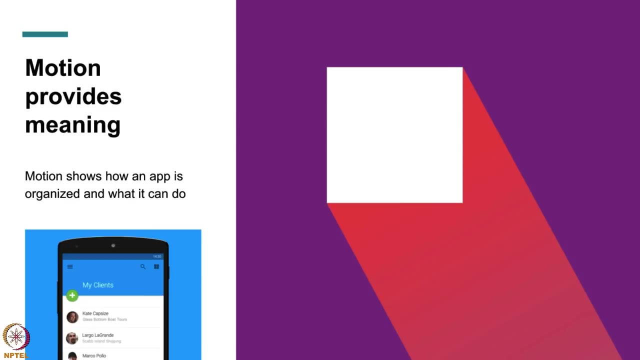 and focus. decisions ranging from choosing the right colors to images spanning from edge to edge, large scale typography and leaving white spaces intentionally help in achieving the goals of material design. the next principle is motion provides meaning. motion in the world of material design is used to describe the shape of the object. the shape of the object is defined by the shape. 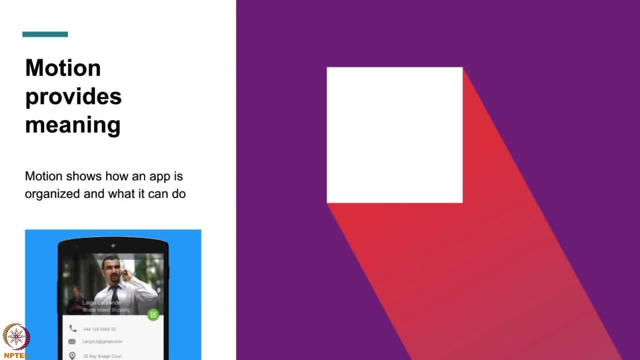 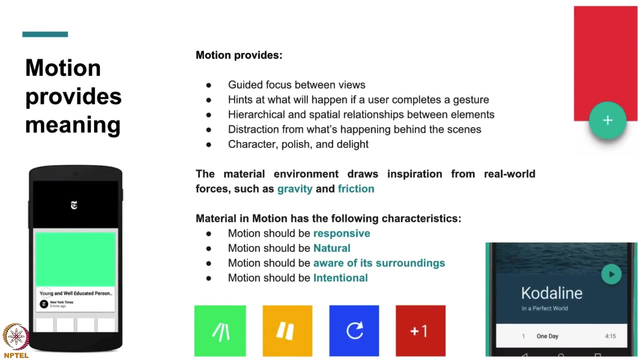 of the object. the shape of the object is Derogatory, describes spatial relationships, functionality and intention butみ. but why is motion important? motion shows how an app is organised and what all it can do. motion provides add精粛. 搞 Ed 강分混在機器上複習用行動。 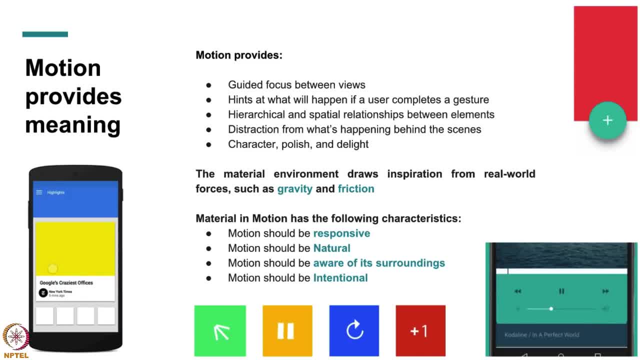 so it tells you where the focus lies, in which view. so whenever a motion is occurring in any interface, your eyes tend to go in that direction, and hence the focus is shifted to wherever the designer wants. the next one is motion hints at what will happen if a user completes a gesture. 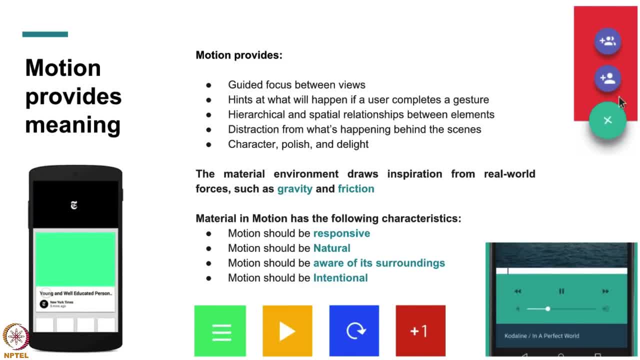 this should be intuitive enough, seeing the motion which is taking place. motion provides hierarchy and spatial relationships between elements, so it makes visible as to which elements are of more importance in a screen and which play a more crucial role than others. motion provides distraction from what is happening behind the scenes, like so whenever any back-end activity is being performed. 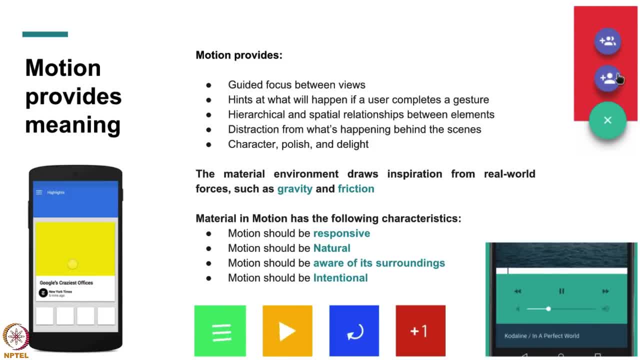 there might be some time lag while the processing takes place. to distract the users from this time lag, motions and animations are needed so they keep the user distracted while any back-end activity is being performed, so it makes visible as to which elements are of more importance. so how does material move? the material environment draws inspiration from real-world forces like 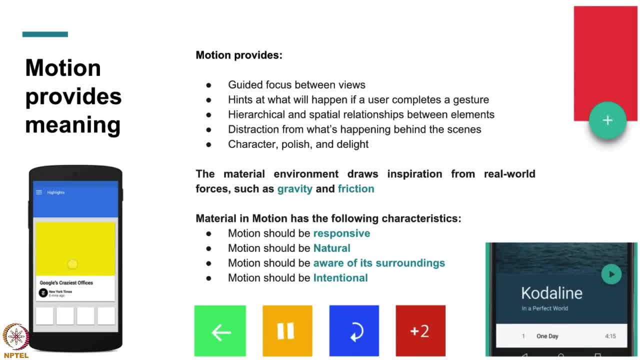 gravity and friction. these forces are reflected in the way a user input affects elements on the screen and how elements react to each other. so a material in motion also has the following characteristics: the motion should be responsive, it should be natural, it should be aware of its surroundings and it should be intense. the motion should be responsive, it should be natural, it should be aware of its surroundings and it should be intense. 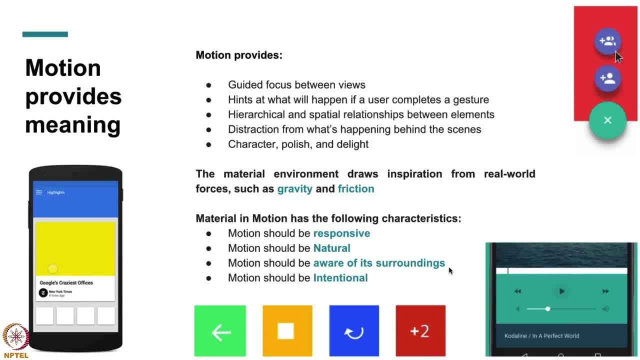 it should be intentional, so material is full of energy and the design should be quick enough to respond. what to whatever is happening. so by what we mean is mean by a natural motion, is the laws of physics should not be violated. the motion should be natural, like forces in the real world, such as. 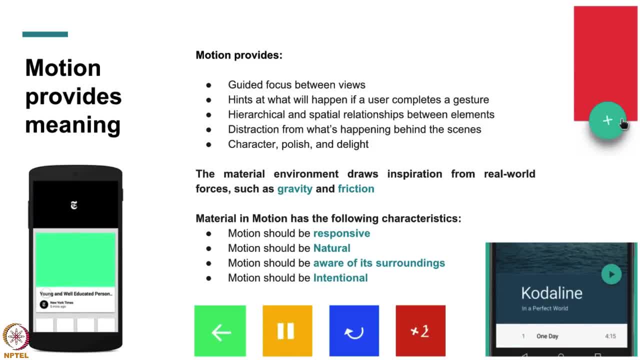 gravity and friction. so what we mean by motion should be aware is material is aware of its surroundings, including user, as well as other material components which are there on any screen around it. so it it the other components should also show how the movement of this particular material is taking place and it should be in synchronization with other materials around it. 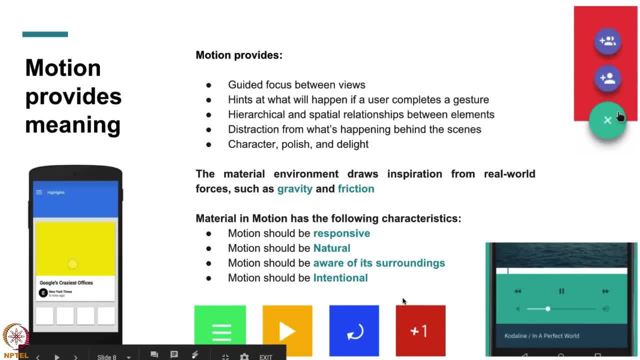 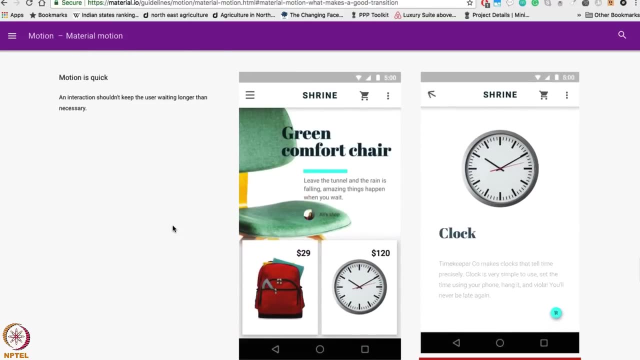 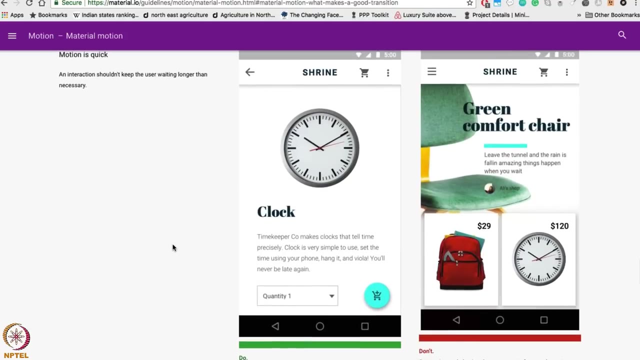 motion should be intentional. material in motion guides focus to the right spot at the right time. the user should be able to focus on the component that is intended by the designer. now we would move to the material design website, which is hosted by Google, and I would run you through some examples of good motion and bad motion. so this is one. 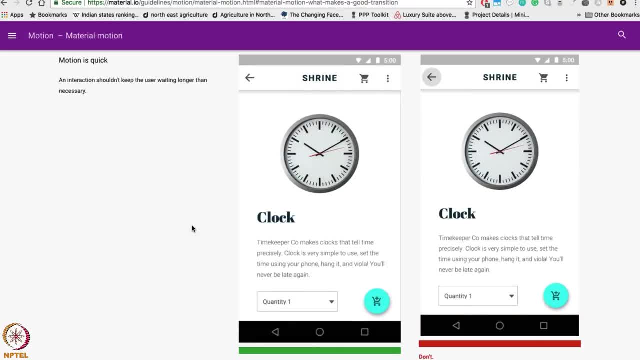 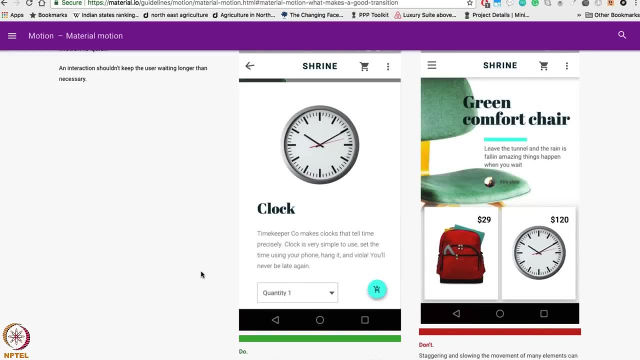 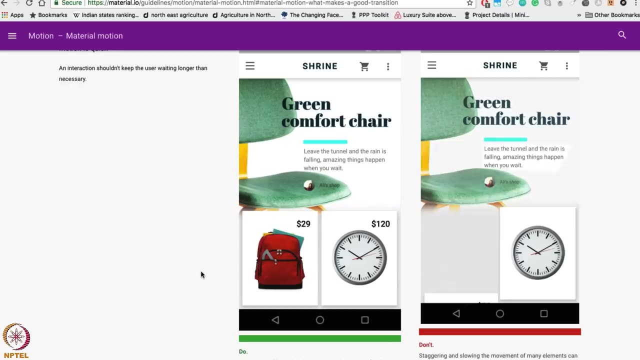 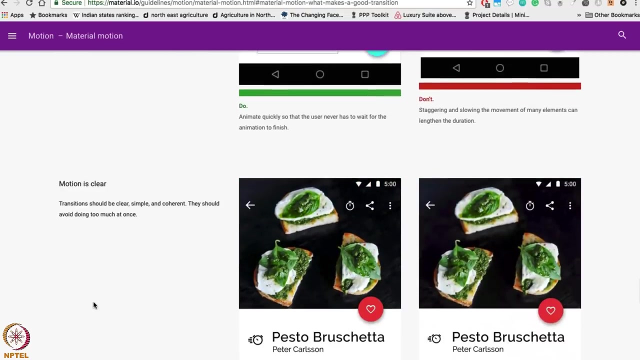 example of a good motion which is portrayed by Google, and this is a bad example. so observe carefully what is the difference between the two examples. so the second example. as you can see, there is some time lag as a lot of activities are happening simultaneously, so that should be avoided. the second feature of a good motion is that the 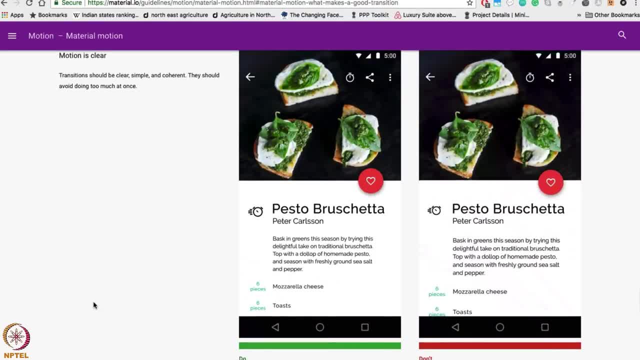 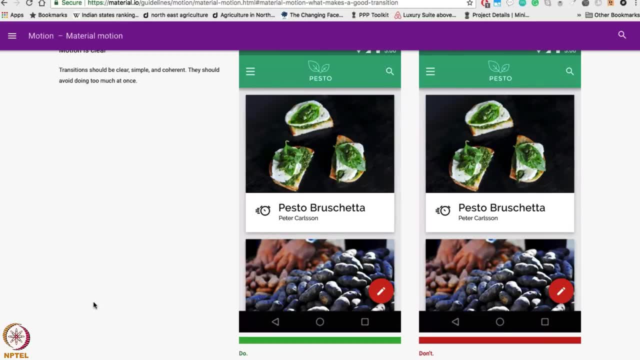 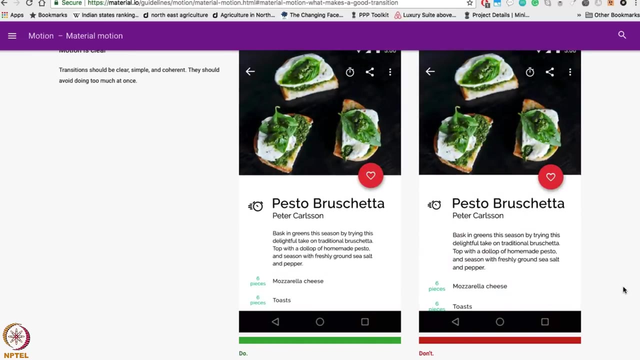 motion should be clear, so carefully observe the two interactions which are taking place. so the first one is a good practice, while the one on the right hand is not a good practice, as multiple elements are moving in different directions and they are confusing the user- what is going in what direction? and they are crossing each other's paths. so such motions should generally 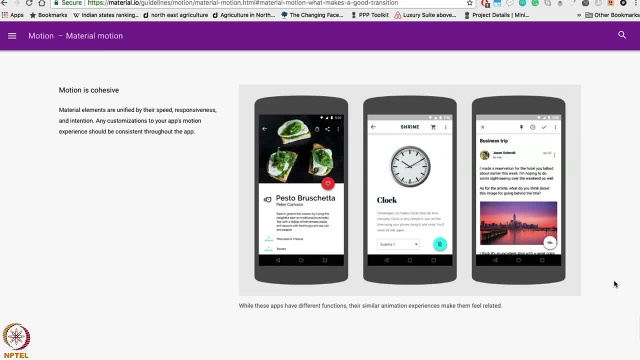 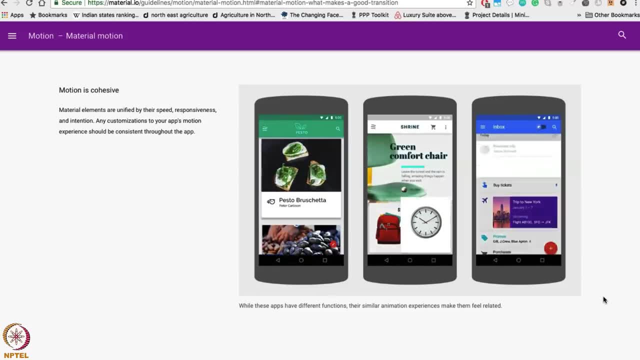 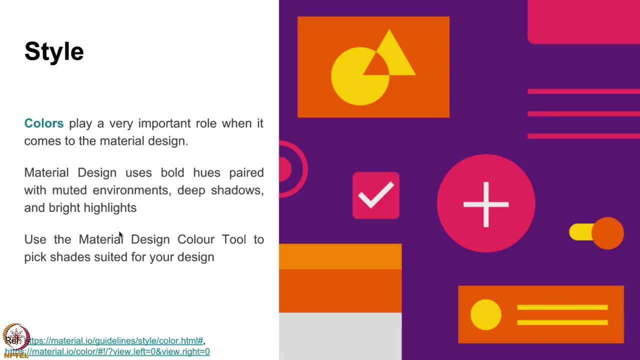 be avoided. and the next one is: motion should be cohesive. it means that if there are multiple components on the screen, they should move in synchronization with each other so that they feel related. so these are some examples of good motions. so next we have the style guidelines of material design. color is the first one. so color and material. 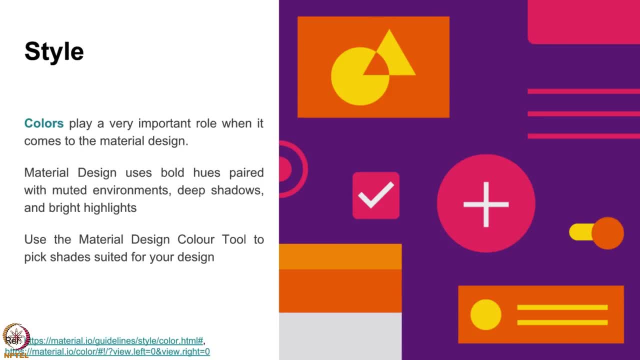 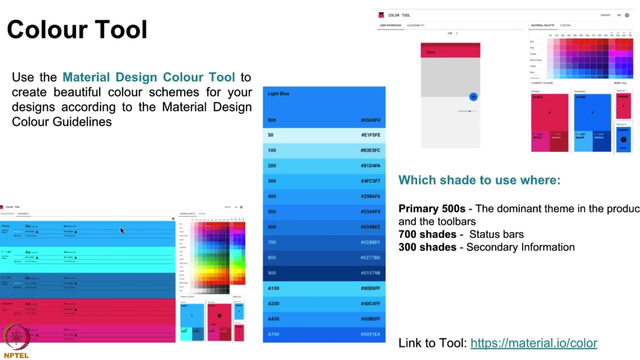 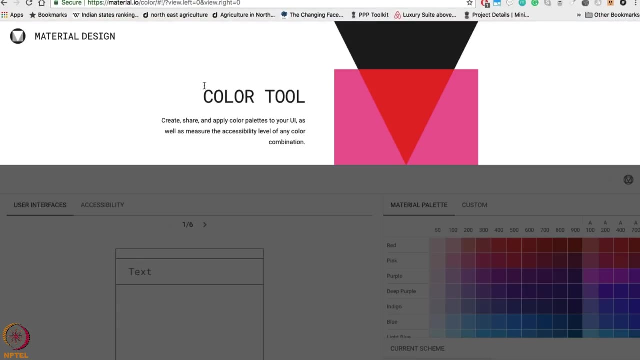 design is inspired by bold shades paired with muted environments, deep shadows and bright highlights. so here are. so now I would tell you how to use the material design color tool, so you can simply go to the link which is given here on the slide. once you go to the link, 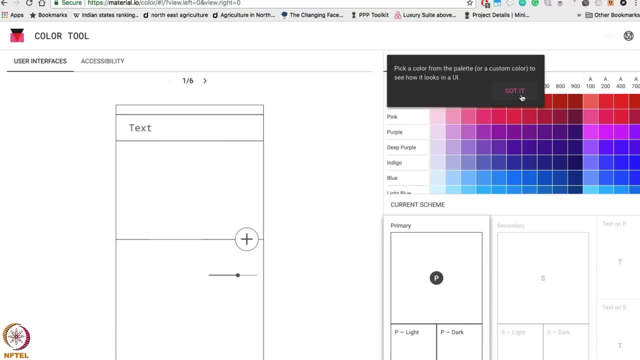 you would be shown an example interface for which you could choose your, you could make your color scheme so you can navigate across different elements as well. okay, so this is the basic. the first entry is point of any interface which is there. so first it asks me to pick the 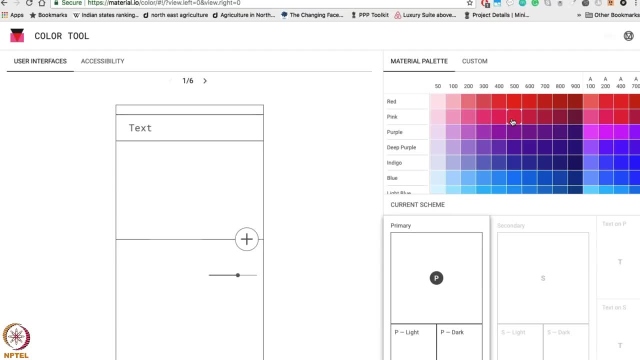 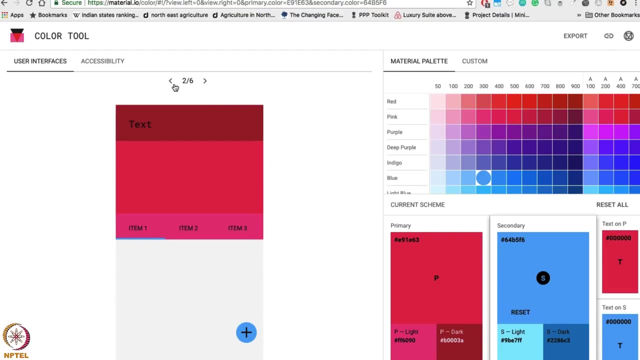 primary color. so usually we choose five hundred SAS the primary color. so this is what I take. next up, I go to the secondary option and choose a secondary color for my screen. so here I am done once. so now you could also see how this, how the selection of your colors, would show across. 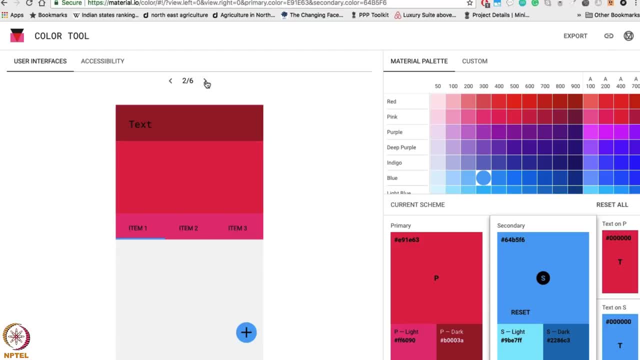 different screens. so here are some preset examples and you could see how your color is settling right. so you can see how the colors are fitting right. so you can see how bright colors are selected. therefore, you have several choices in your screen. greater Espia color with colors, for example, if 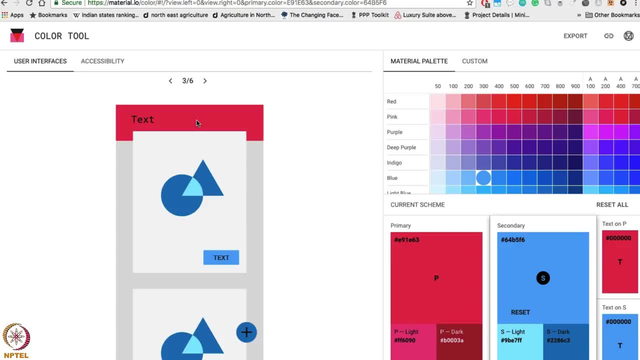 like, for example, you touched engineers. when you touched ITM, you saw two colors. någonting color scheme would look once your app uses it and how different components would show it. so once you are satisfied with the color selection, you are free to choose whatever you want. 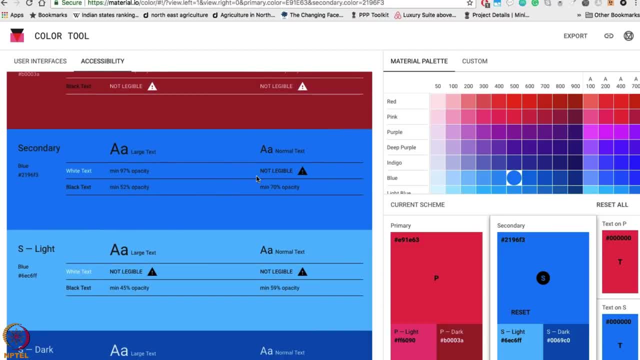 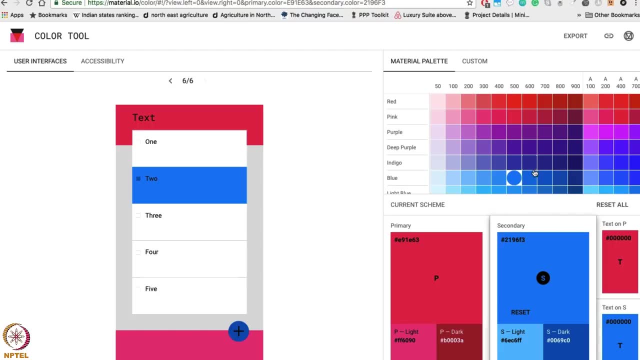 so you could read more details about it, whether the colors are legible or not, so it shows you the accessibility options. so once you are satisfied with the color scheme of your app, what you can do is you can go to the export option and say: if i'm developing for android, click. 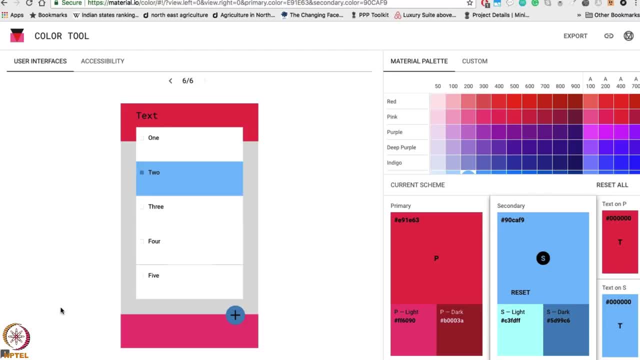 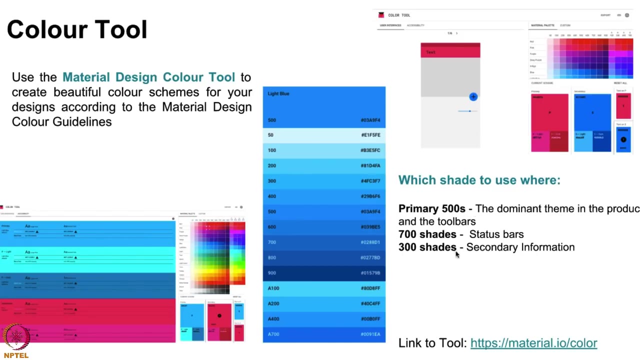 on this, so the colorsxml file would be downloaded and this can directly be imported into android studio and that color scheme would be used for your app. so this is how you can use the color tool for material design. these are different shades and different guidelines that you have. 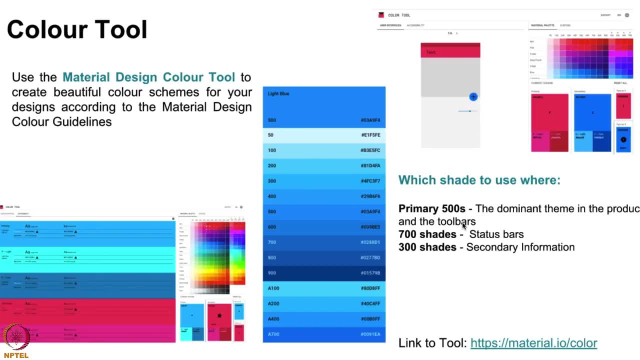 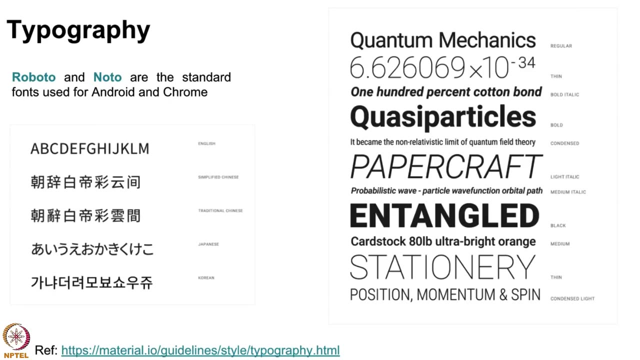 so usually the 500 series shades are used as the primary colors and for the toolbars, then the colors with the 700 series. they are used in the status bars and usually the usually the 300 series is used for the secondary information. so next up we have typography. so basically roboto and noto are the two standard fonts. 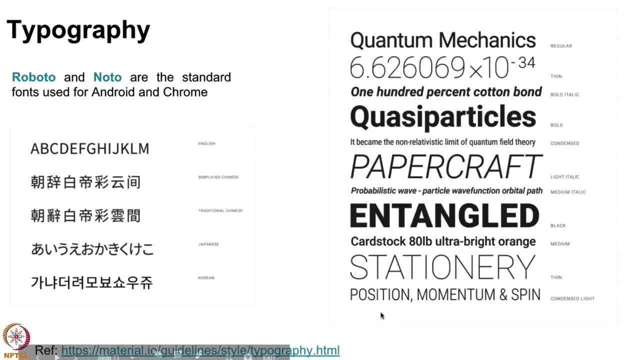 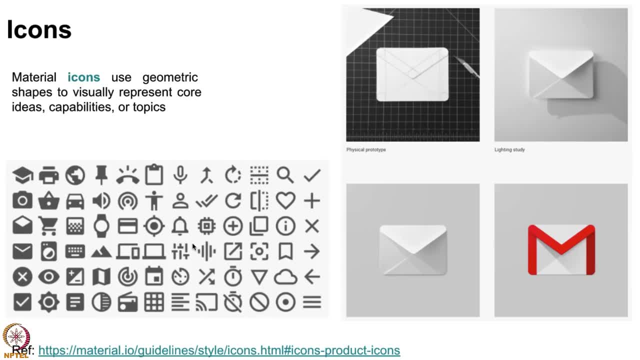 which are used for android and chrome. you can read more about these fonts on the link given below. so next up come icons. each and every icon in the material design library has been crafted very has been crafted carefully. so each and every icon has gone through a very rigorous cycle. 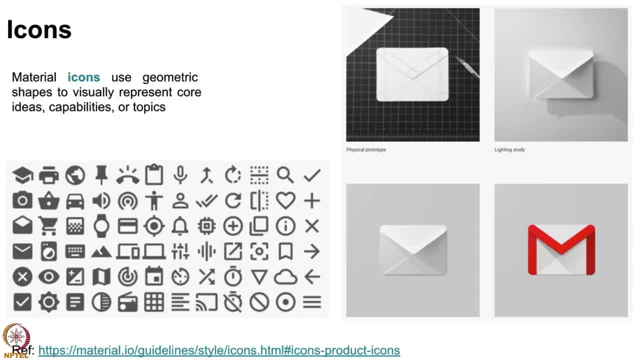 of designing before, which i would act with before it is actually given out for usage. so a product icon design is inspired by the tactile and physical quality of material. each icon is cut, folded and lit as paper would be, but represented by simple graphic elements. the quality of the 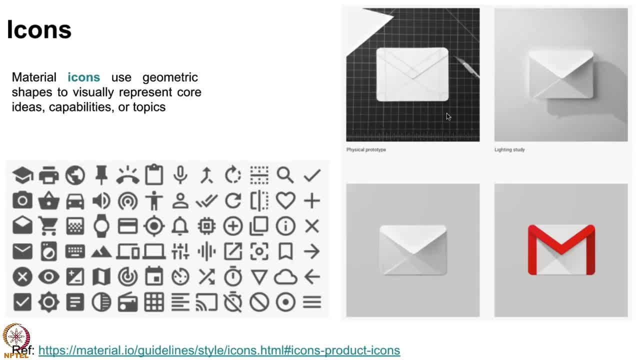 material is sturdy, with clean folds and crisp edges. so in this example, you could see how the logo, how the icon of gmail, has evolved. they have. they have actually taken paper and crafted it into the probable icon that it could be. they have studied the lighting and shadows of it. 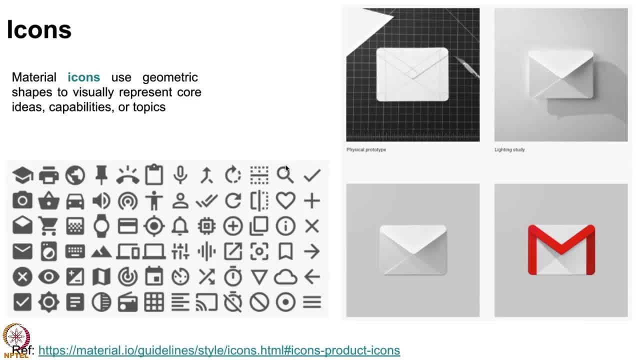 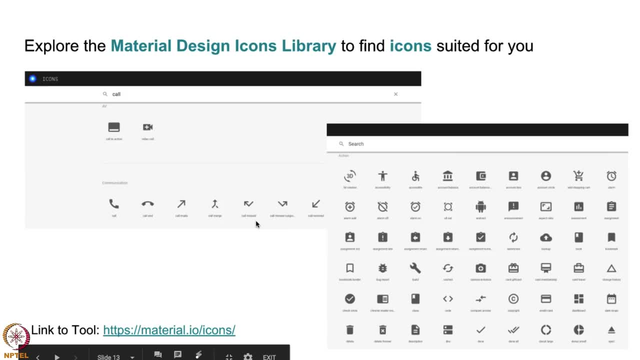 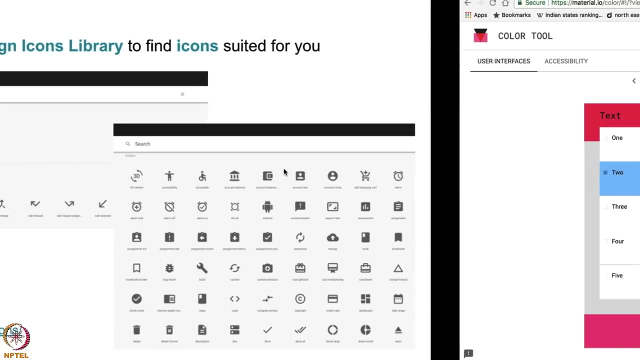 and then they came up with the final prototype. so material design has a very good collection of icons that you could use. so here's the link given for the icons, and it has a very good search functionality from which you could choose whatever icon you want. so i'll show you how to use and pick icons for your app. 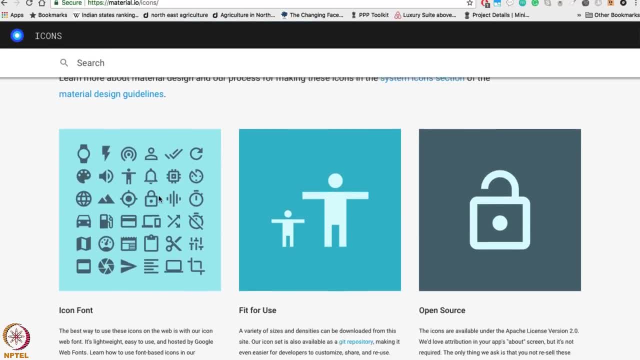 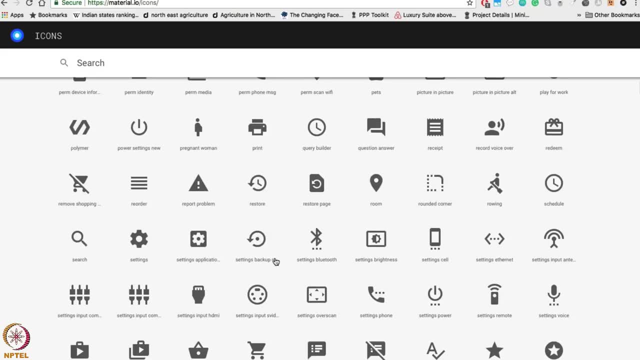 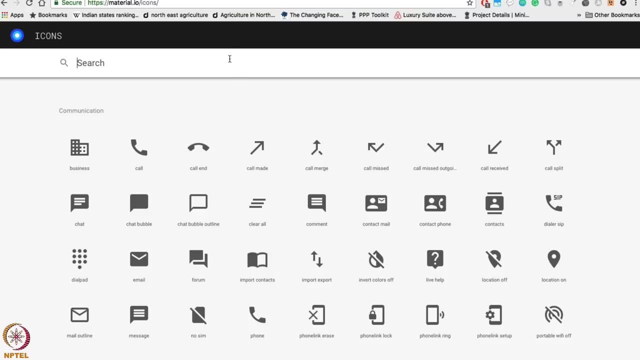 so go to materialio icons and once you go here you would be able to see different icons which are available. so you have a wide variety of icons that you can use from different categories. so, say, i'm making a calling app, so i'll just search for icons which 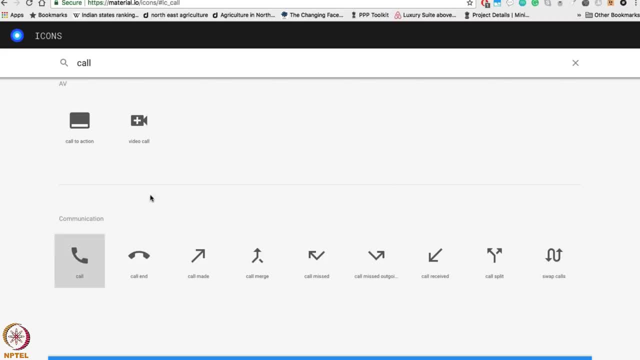 depict calls and i would be able to choose them, and then i can simply download them in whatever format i want- say, i want a png- and the download would start. you could even choose the color scheme- whether you want it in white or black, and you could choose the size of the icon from here. 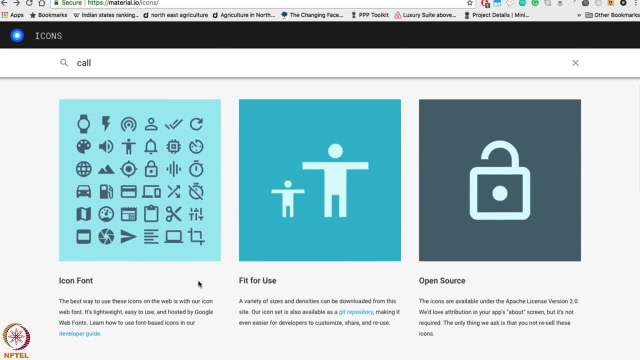 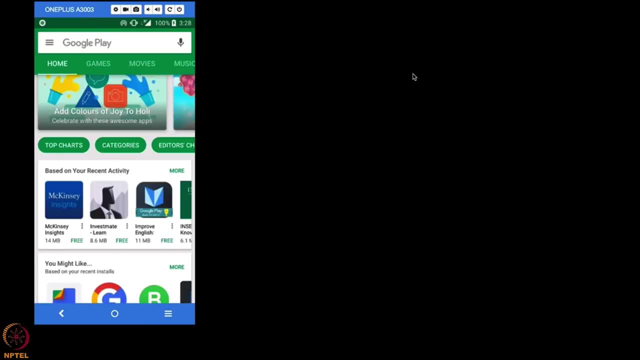 so this is how you could download whatever icon you want and use it for your design. hello, now that we have seen the basics of material design and the basics of metal design paradigm, let's just have a look at some of the real world apps and see how developers use these paradigms. 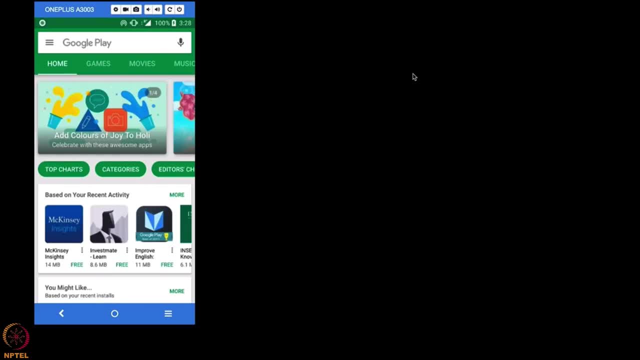 and incorporate them in their apps. so let's take the example of google play store, like you can see on the screen, to understand some of the basics of material design paradigm. I'm sure almost every Android user must have used this app at least once. So, looking at this app, if I look at the home screen of this, I can see there is a lot of 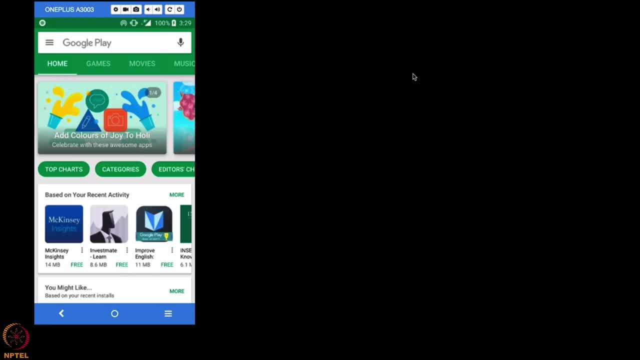 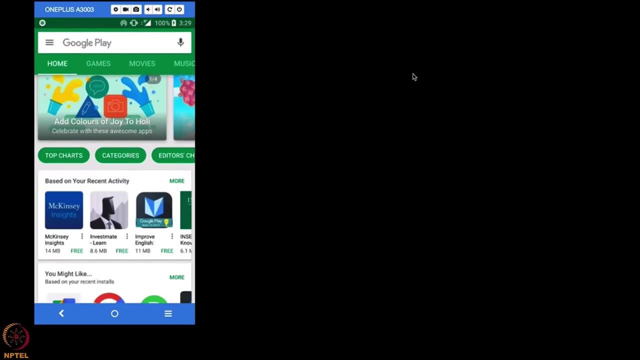 graphic content. There's a lot of bold graphical content. You can see some shadow lines here on this card which says add colors of joy to Holi. You can see some shadowy outline to this box. Now coming to the color scheme which, as Simran said, is a very important part of material design. 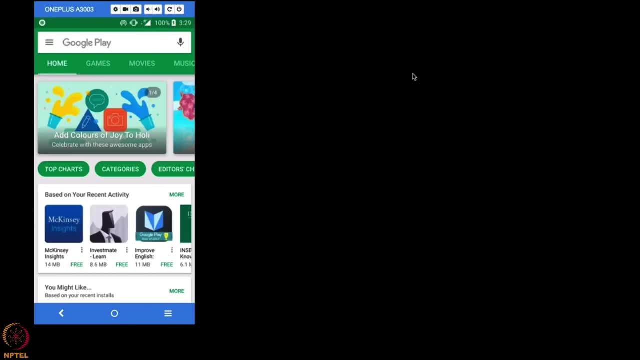 You can see that. first, it is consistent throughout the app. You can see green on the top mode tab. You can see green here for every icon, Green for text. So one thing we see is consistency. Second thing, as far as using the shades of colors is concerned, 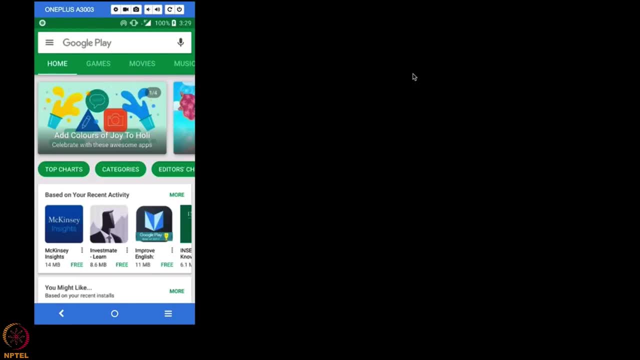 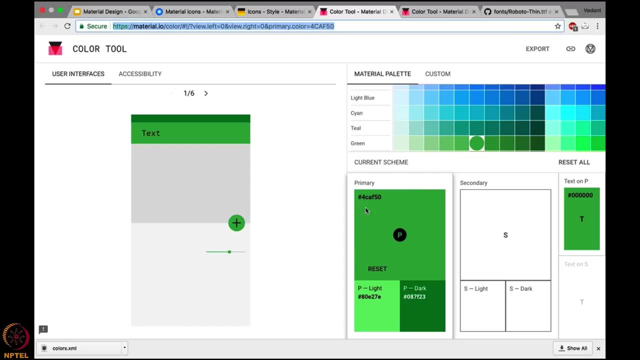 we saw that the shade corresponding to the number 500 is usually used for different books. so when you look at the library we were able to see the code for a separate copy of that for primary. so if you look at Google's color shade we can see that the primary. 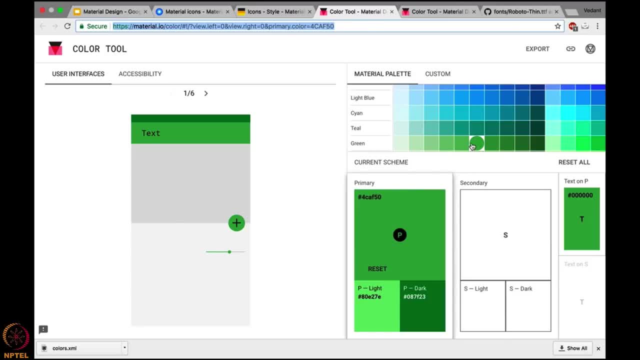 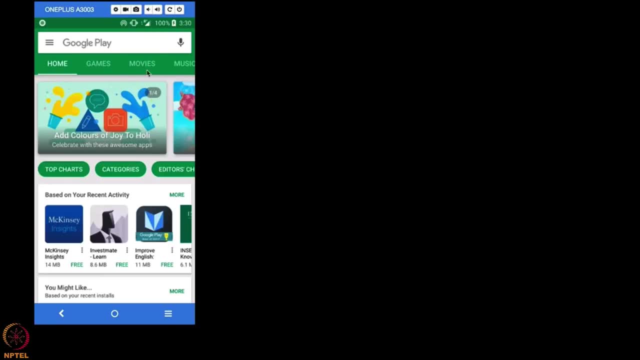 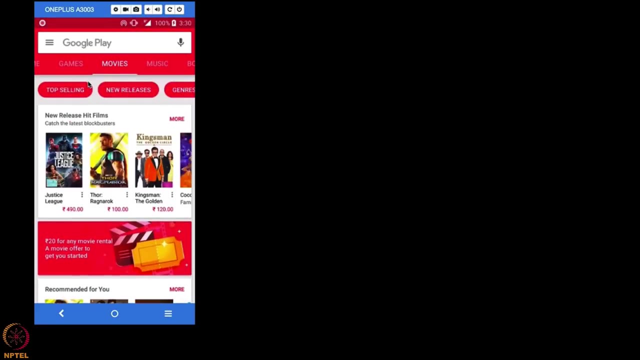 shade, the, the 500 shade corresponding to green, is the one which is exactly being used by Play Store as well. now, moving to a different tab, let's say movies. we see that the color has changed but again, it's consistent throughout and again, if we want to have a look at the shade of this color, we can see that this 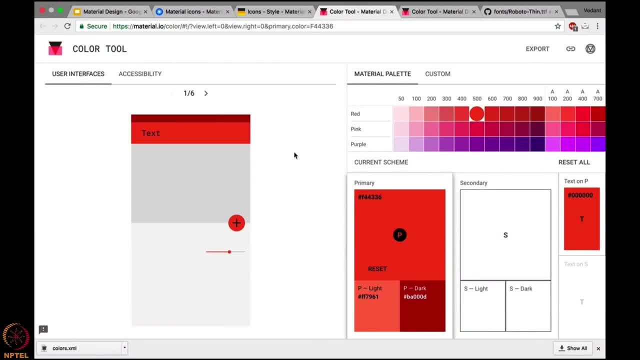 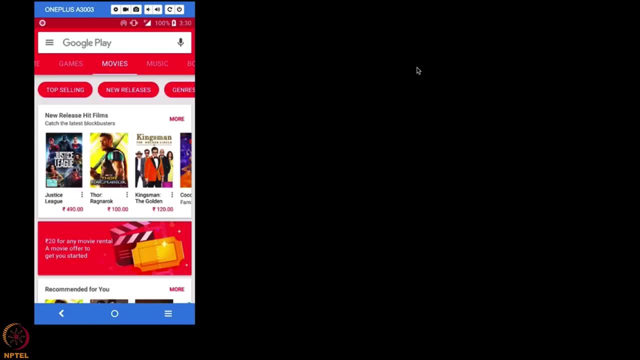 corresponds to the 500 shade under red. this is this is exactly what Google is using as well. so color is consistent color. the shades are rightly used. content written on top of any colored element is legible and a lot of graphical content is there. another thing is font. so the font used by font of the 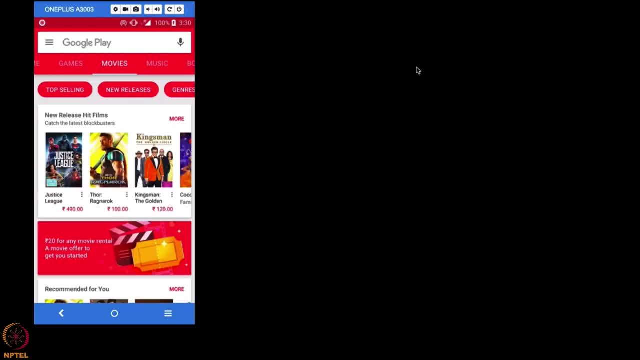 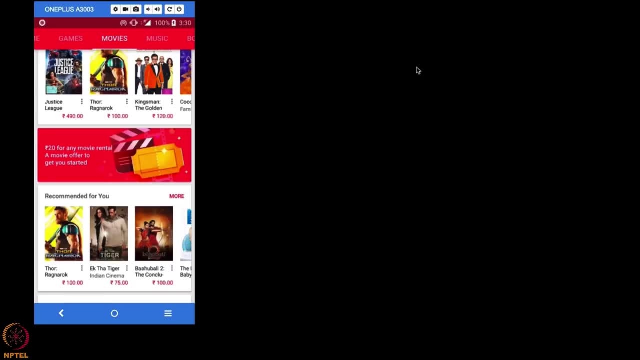 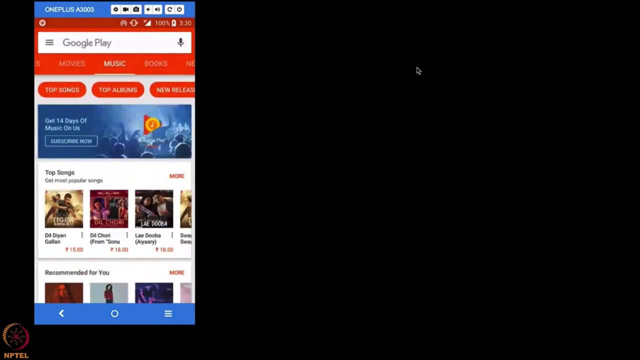 typography, like Simran said. so font used by Google Play Store is something called as Roboto and this is a formed developed by font developed by Google, and you can see that this is again consistent throughout the app through every tab has the same font color might change, but font color color of the tab might change with the font. 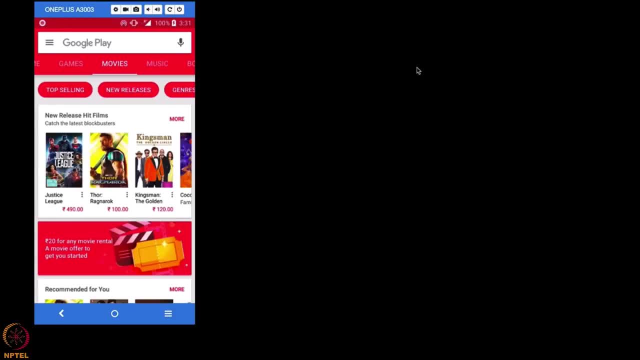 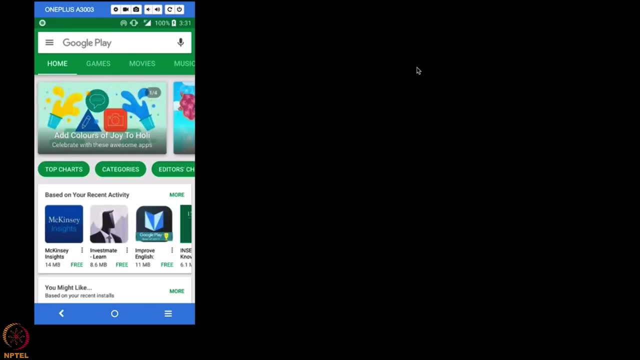 color and the font itself does not change. now, another very important thing of material design is the way things move around. it should be intuitive. it should, it should be. basically, a user should be able to yeah, yeah should not have to figure out how the movement is. it should come naturally to. 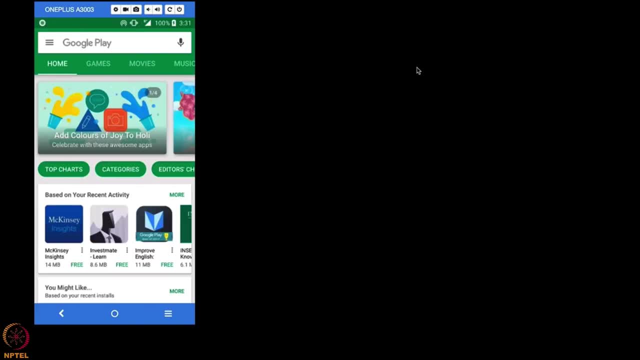 a user. so, looking at this app, the first thing i can see is the first card which i see. i see a small part of another card, so intuitively, i would try to slide left to see the next card. and that's exactly what i do: to see the next card. 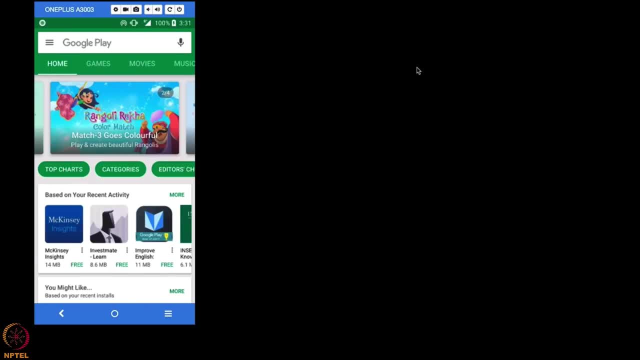 so the motion is smooth, the motion is intuitive. again, if i want to scroll down, it's all very smooth, it's all very intuitive, it's it's it's basically enhancing the user experience as a whole. so that is another very important thing which we see in almost, which is a very important element of 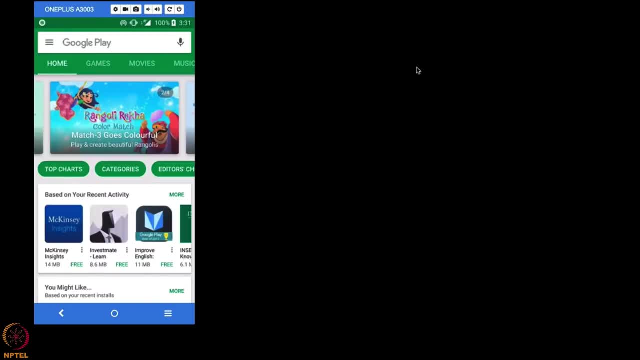 material design and we see it in almost all apps we use. uh, another thing which simran talked about are the icons. so google has made a lot of icons under the material design category available to the public and you can see some of these icons. even they're using some of these icons, like 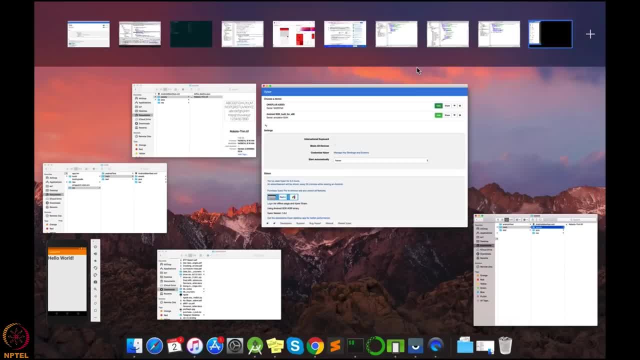 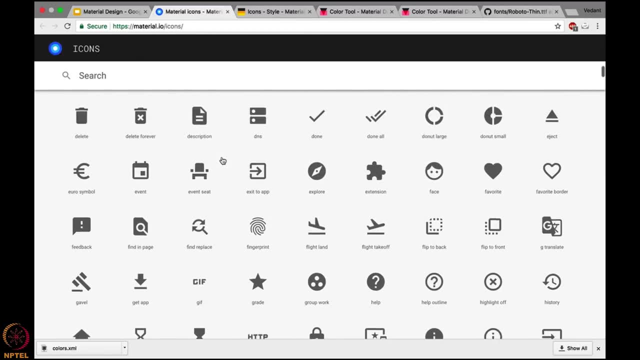 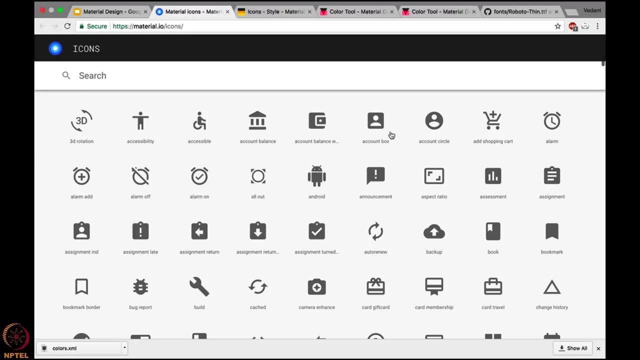 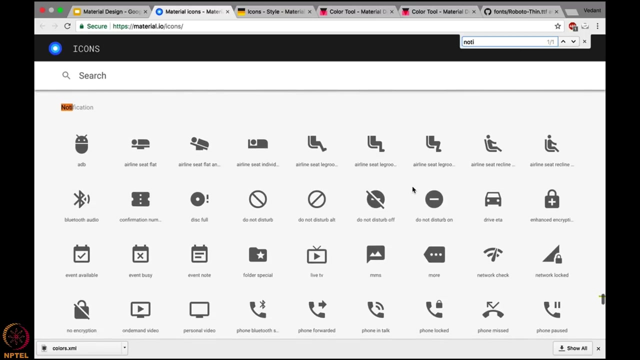 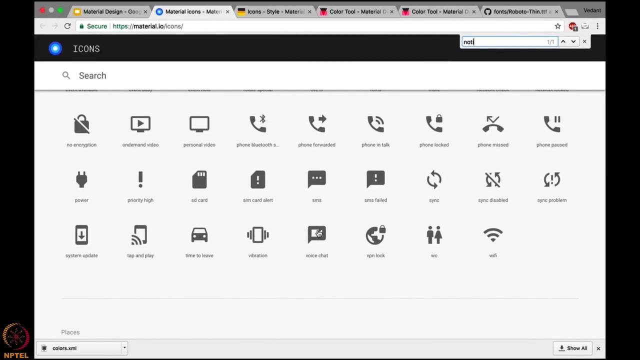 notification, account settings- all these can be found at this place. so materialio icons you can see probably, yeah, so you can see like the account one, account circle, account box, and probably you can see notifications, yeah, so, yeah, basically all these icons are available here. okay, so now, if you're familiar with android app development, you 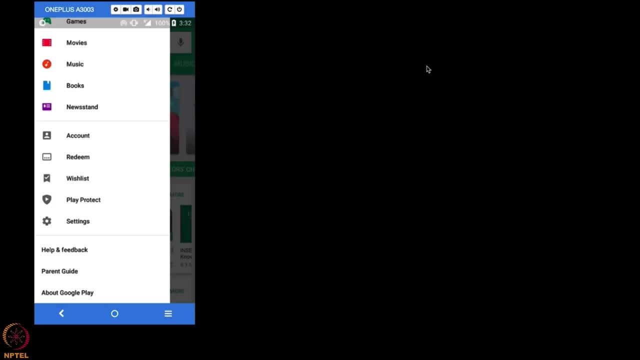 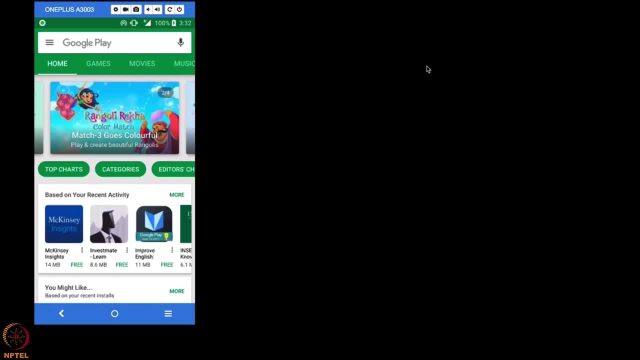 must have wanted to use these elements in your app, or you must want to. you must need to use these fonts and colors in your android app or the rn ios app which you're developing. so let's just quickly see how we can actually incorporate these colors, or. 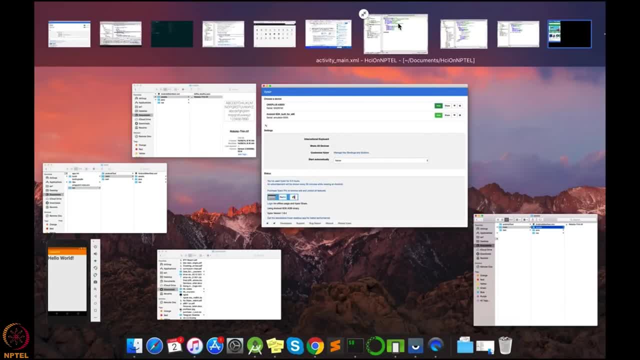 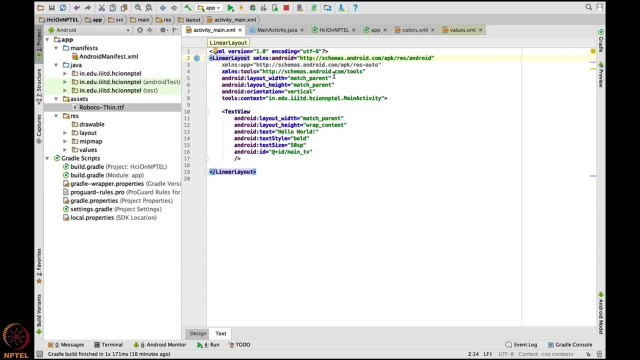 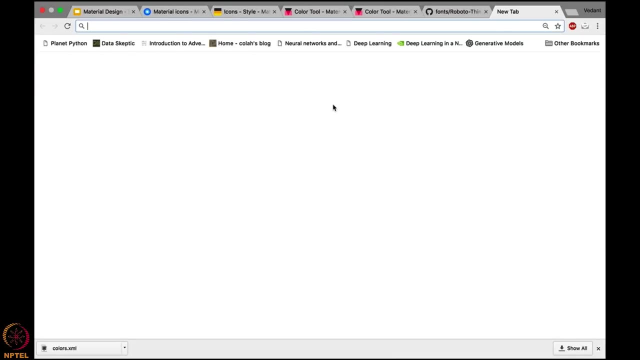 these fonts in our app. so for this you're gonna need android studio, which is a very famous framework made public by google, which allows users to build android apps. so just download google play store from google's website. i think they have a lot of great apps for you to use and you can download it from google play store. 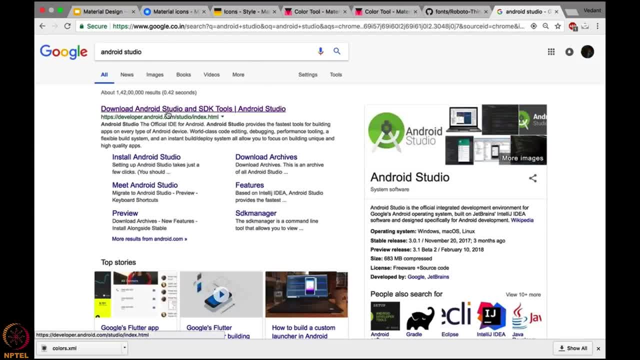 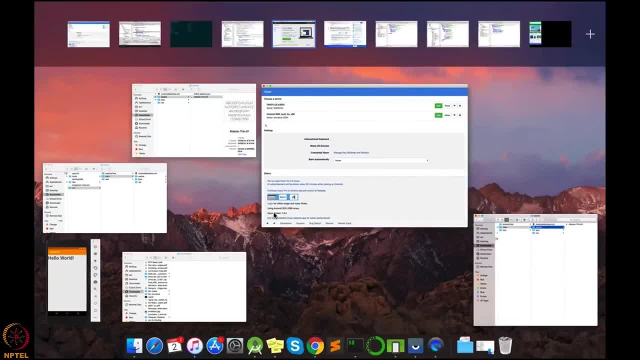 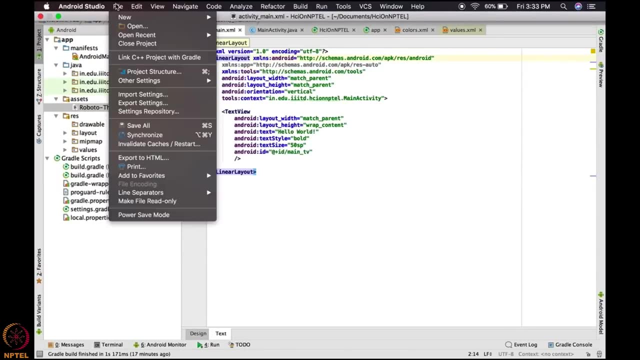 and you can also download it from google play store. yeah, so from developerandroidcom. you can download this and install it. so it's all pretty. yeah, just download it and install and once you install, just open it. open android studio and just click on go to file. new new project. 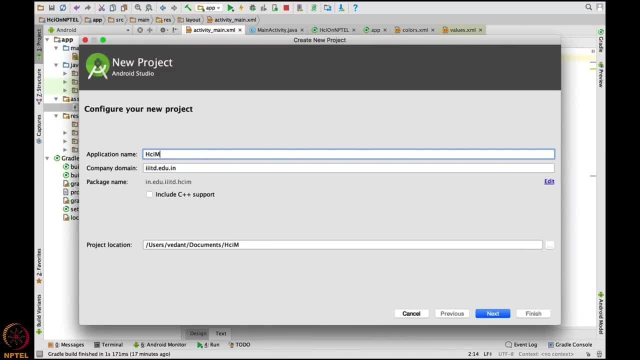 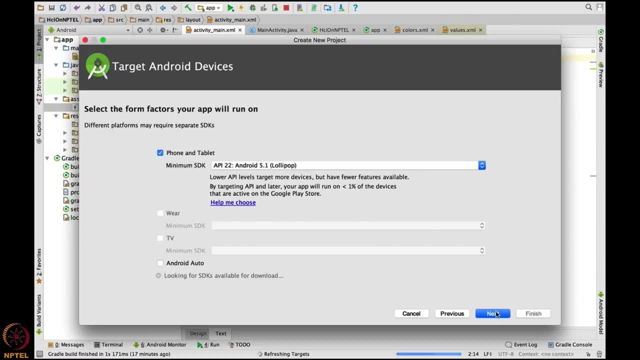 just give it any name. let's say i'll just call it hci, mptl. specify the folder. do next. you can specify the minimum android version your app should be accessible to, so you can set it to anything you want. i'll set it to lollipop, which is. 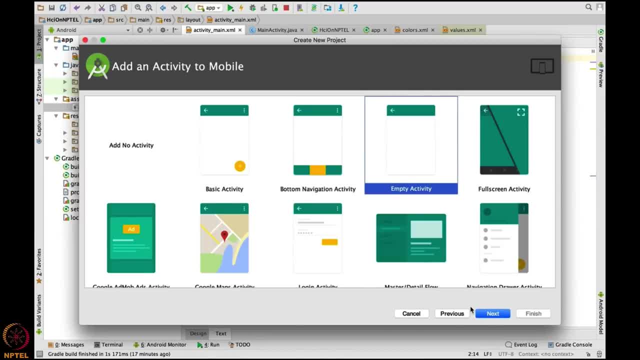 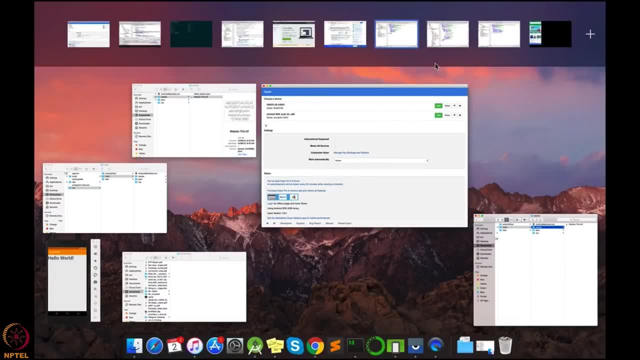 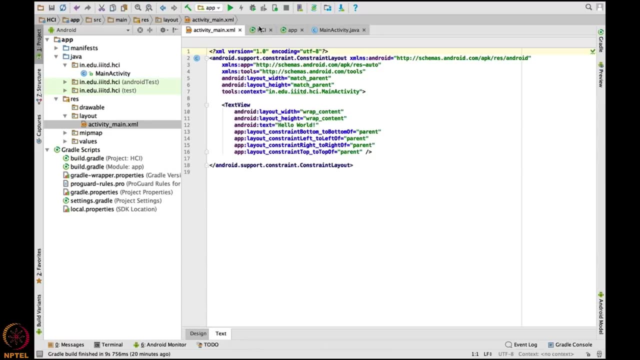 epi number 22.. choose the empty activity. do next. let it be main activity finish and android will then build the app for you. i've already done that, so i'll open that. yeah, so android will build the app for you if it throws any errors. you should. 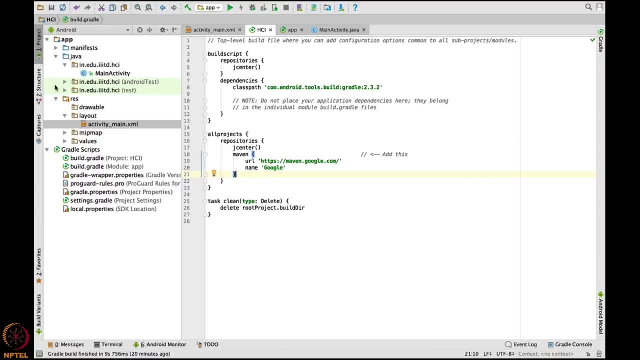 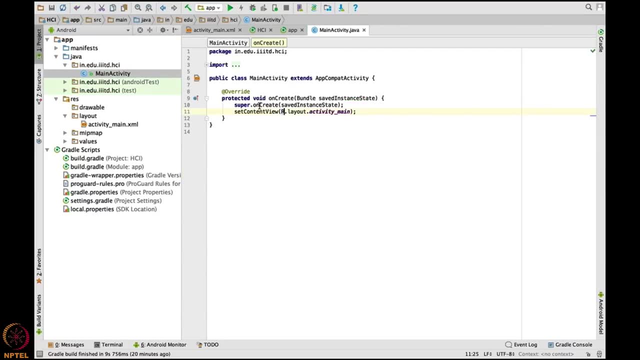 probably. you might probably want to just open, all right. so first i'll go through the layout on the left. so this contains all the java code. this is the main activity. so this is the backend of your app. when you go to res folder you can see a folder called layout. so layout contains how your app looks. so 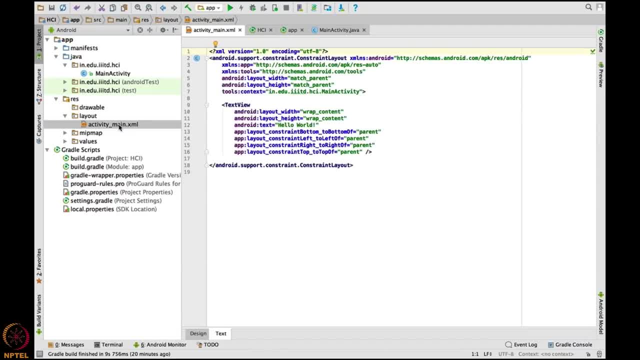 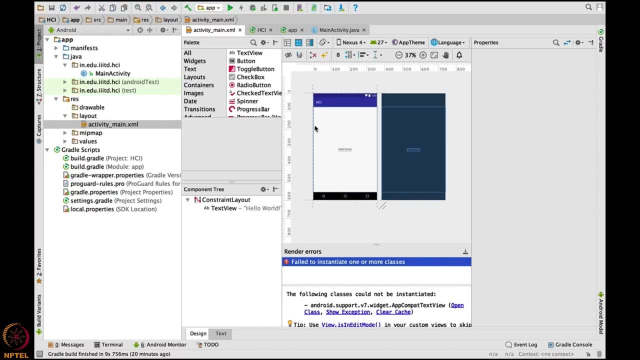 like the name suggests, it's the layout of the app. so my first screen, this is the xml and you you can actually click on the design tab to see how it actually looks. so this, this is the current look of my screen. it will just show hello world and the name of the app on the top, and this is the color scheme. 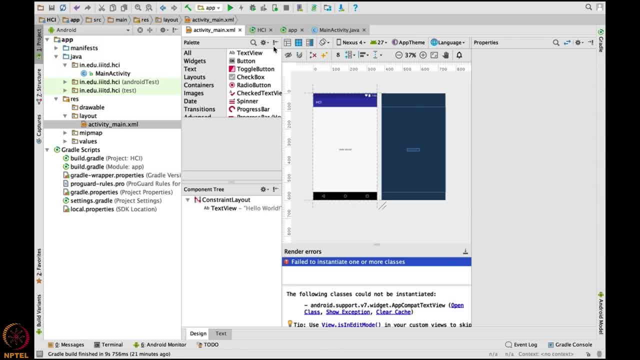 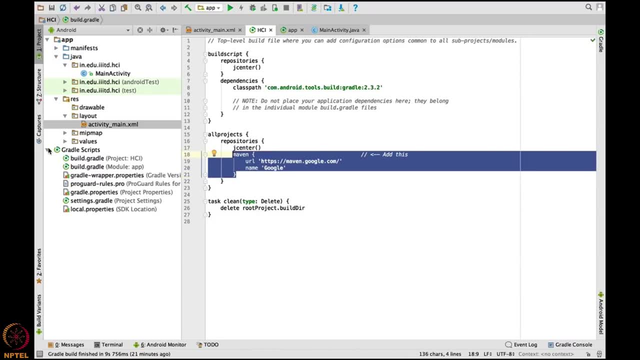 being used. all right, so again now. so if your app throws any errors while building, just put this thing in the gradle app. so this is the gradle file. under gradle scripts, go to buildgradle, open this file, just copy paste this. the error should hopefully go away. all right, so coming back to the design part of it, 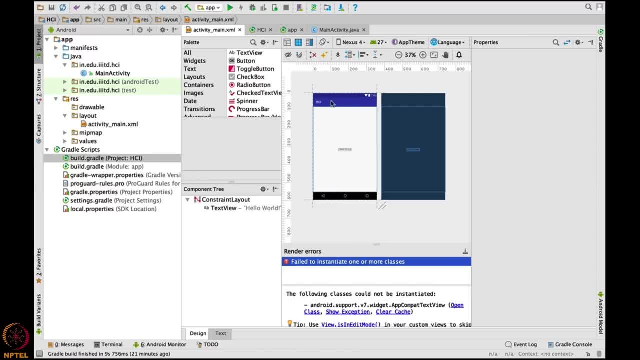 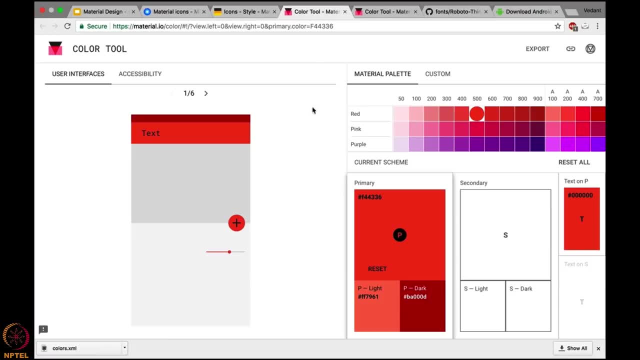 now let's say you want to change the design scheme of the app. blue is not what you want. so let's say you want let us choose something from what google has given us. yeah, so let's choose this color. let's say, or let's say: let's choose orange for that. yeah. 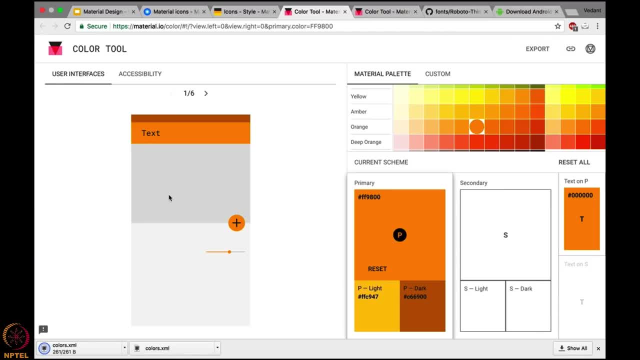 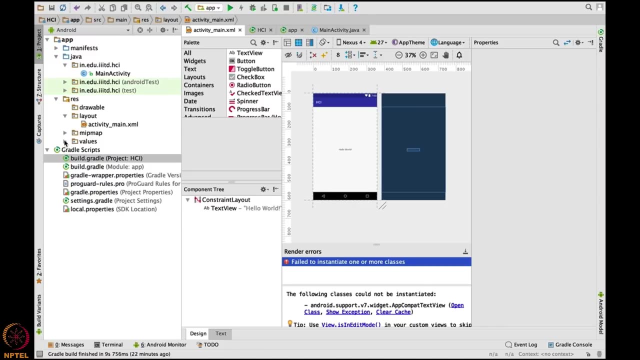 so click on export android. it will download the color for you. now what you need to do is place this. it will download a download an xml file for you. so what you need to do is go to your app. on the left hand side, you can see values. under the res folder, you can see values. 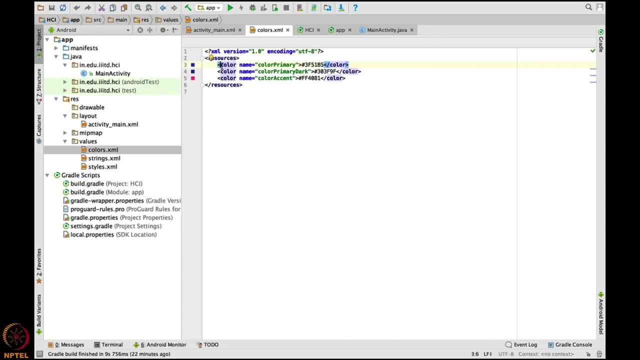 click on colorsxml. so this, this colorsxml, is a very important file because this defines the theme of the entire app. so any color you specify here as primary will be set as the primary color for the entire app or for the entire. basically, you can control it's for the entire app or the entire tab, but for the current 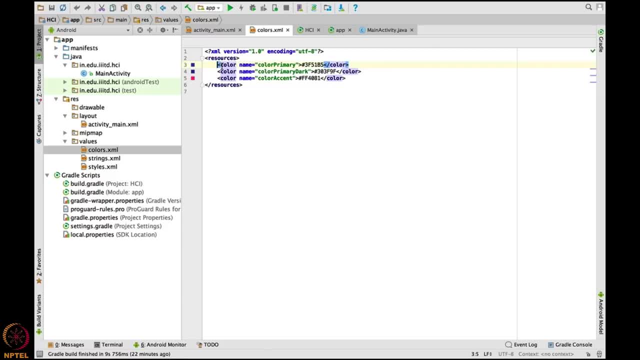 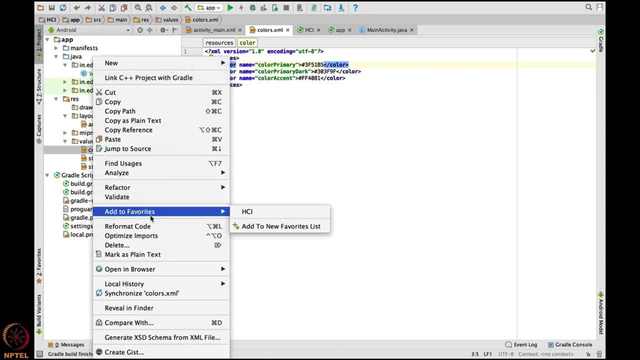 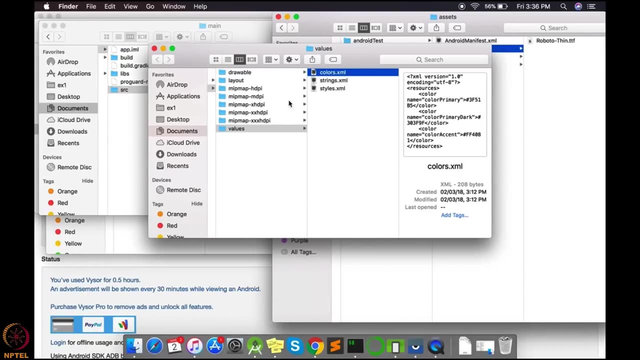 view. this will be the final color, so this is a very important file. so just replace this file with- i'll just keep this for it so you can do a reveal and finder. this actually points you to the folder where it sits- and just replace with the file we. 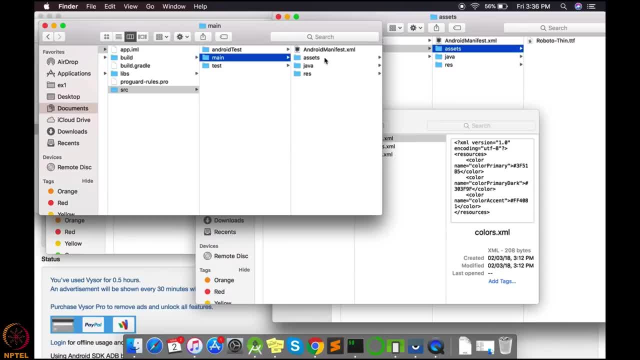 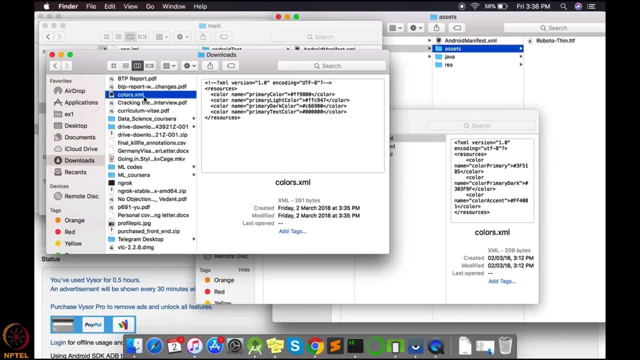 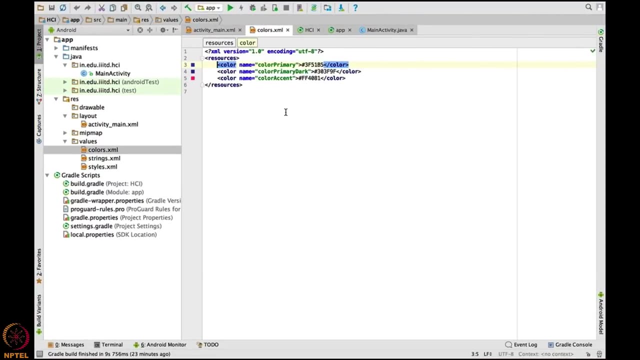 downloaded. so if you're interested, you can click on this. so this is the file we downloaded, just to replace it and click on replace. so now, when you go back to the app, you see things have changed. all right good. so technically now the app should work a. 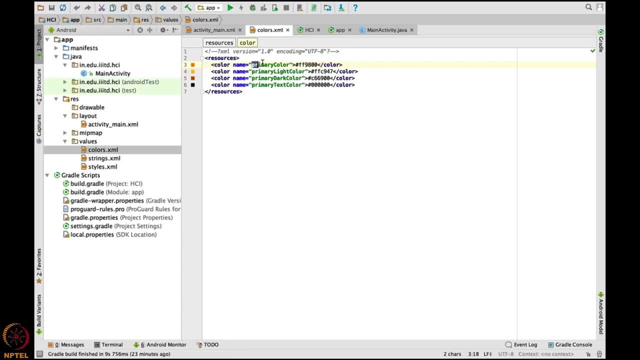 very different color, so let's just see if that works. the colors were different so we might have to change that. So it was color primary instead of primary color. So let's make it color primary. and there was color primary dark And there was color accent, So color accent basically means it's the text color Again. 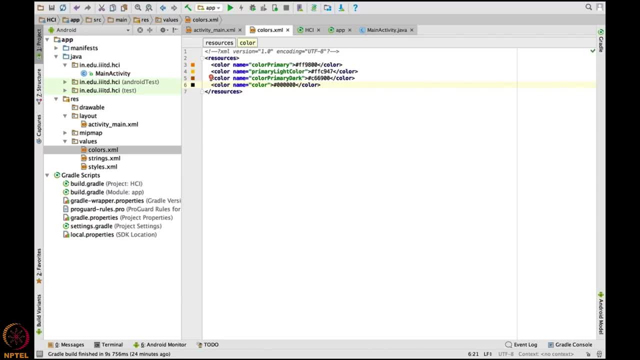 this might not be needed if you're using Android 3.0, which is the latest Android Studio 3.0, which is the latest Android Studio version. My version is a bit old, so probably that's why I have to make these changes. Color accent: this defines the text color And let's just. 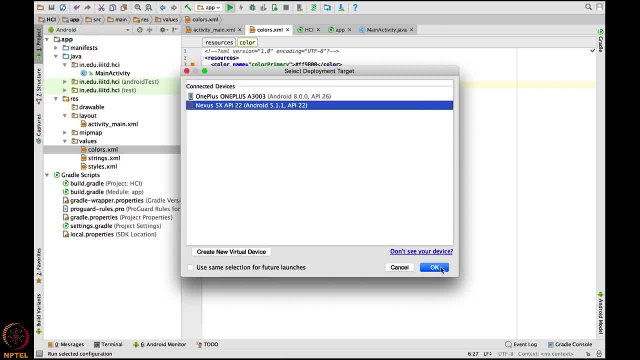 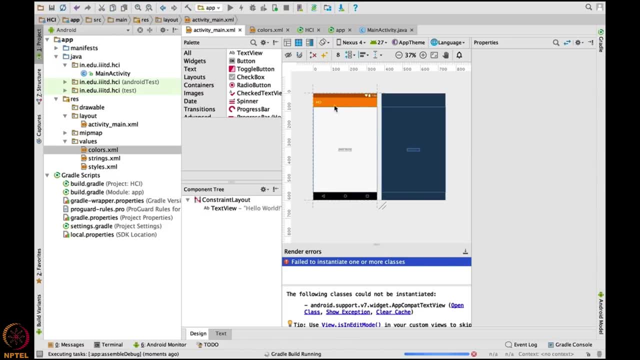 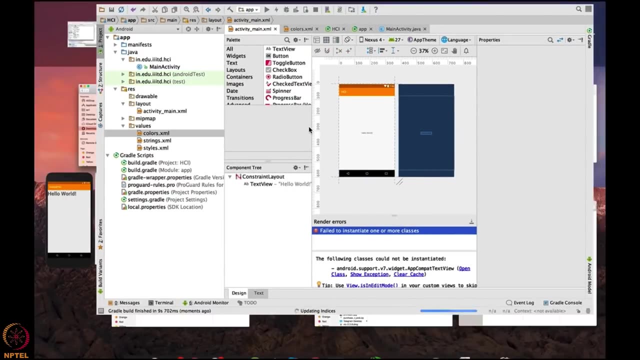 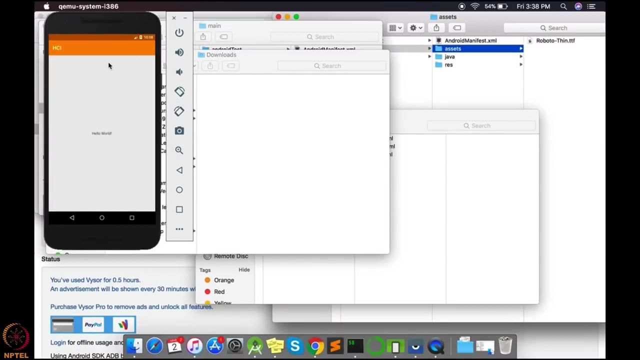 see if this runs now. Okay, So this is the virtual device. Yeah, So you can see. these color changes are reflected in the activity mainxml, which is the layout of my file. Okay, Cool. Okay, So the app build. and okay, great. So we changed from color blue for it to be orange. 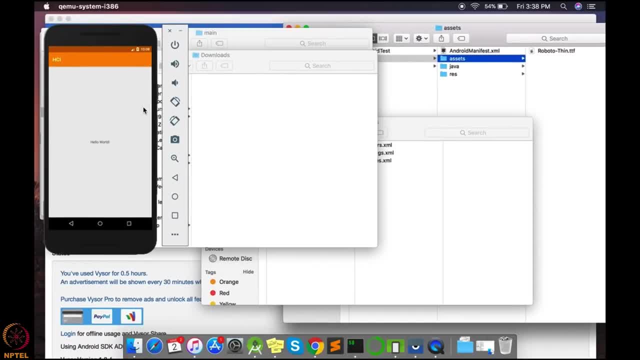 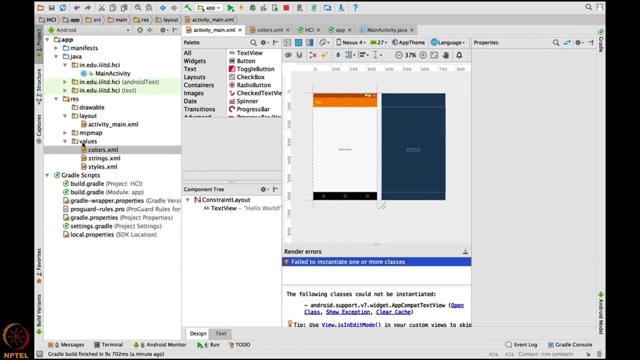 So that's how you change the color scheme of the app Again. if you did not understand, that's fine, because this is more of the Android side of things. I'll just quickly go through it again. So you had values, So there's a values folder under res. Just download the. 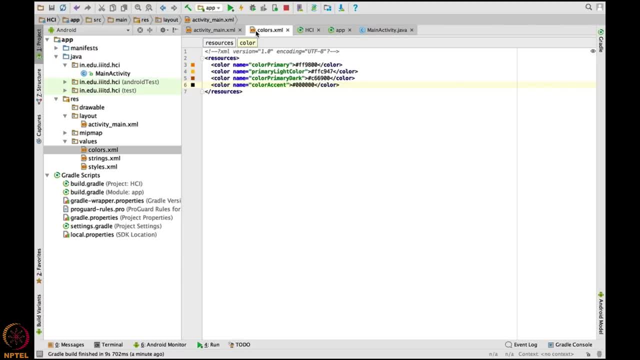 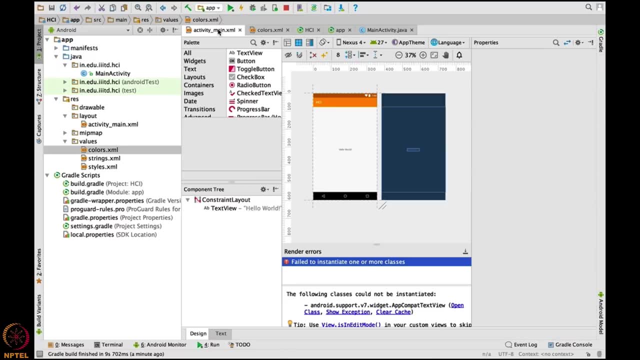 colorsxml, Replace it with the file given here and just go through it again. So you'll see that you can just accordingly, whatever your old colorxml had the names, just name it accordingly And you will see that the color scheme of your app has changed. 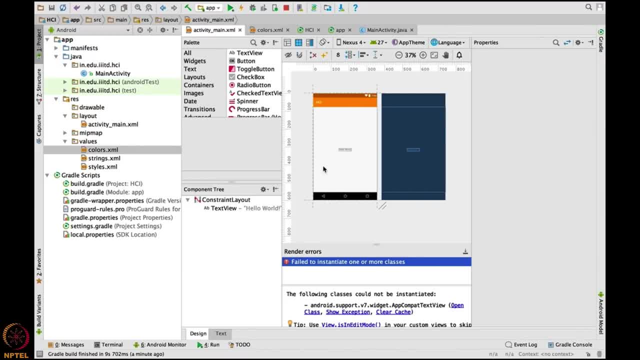 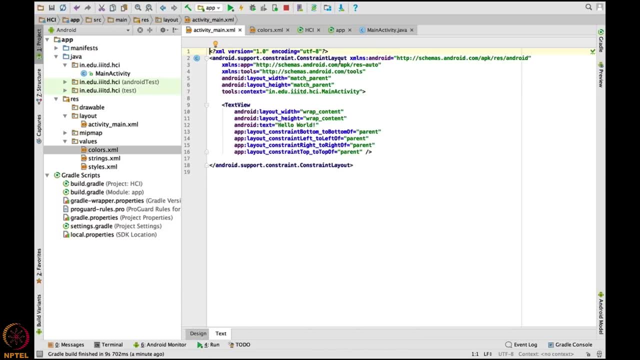 All right. So now, looking at this, I would probably want to, let's say: next thing which we want to look at is font. So if I go to the XML part of this, I can see that this, the font, is the basic font, whichever it was built in. So let me try and change the font. 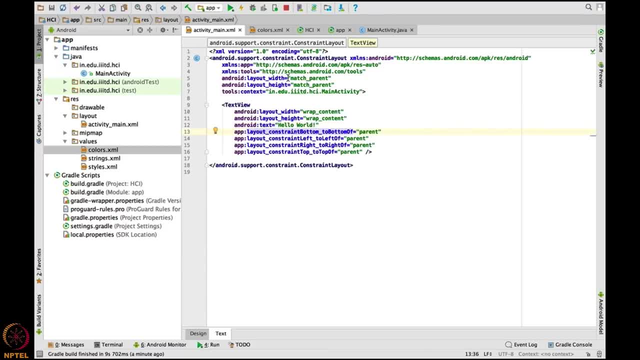 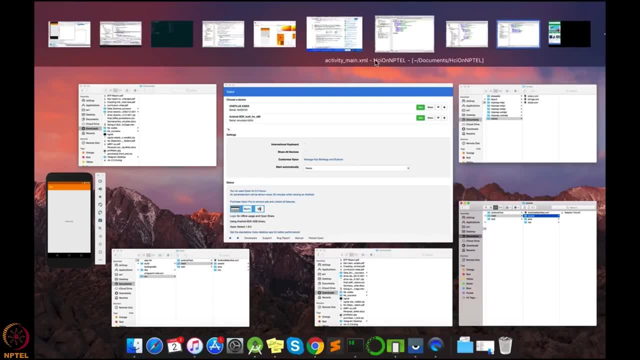 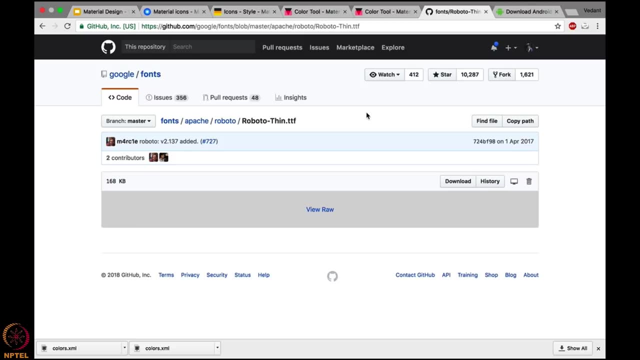 The font of this. So to do that first I have to download a font file. So Google has a file. So, like I said, report is a font which Google came up with And, let's say, I want a thinner version of it which is a little more elegant to look at. You can actually go to GitHub and 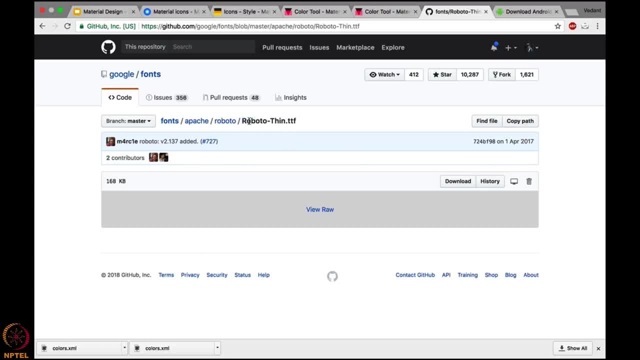 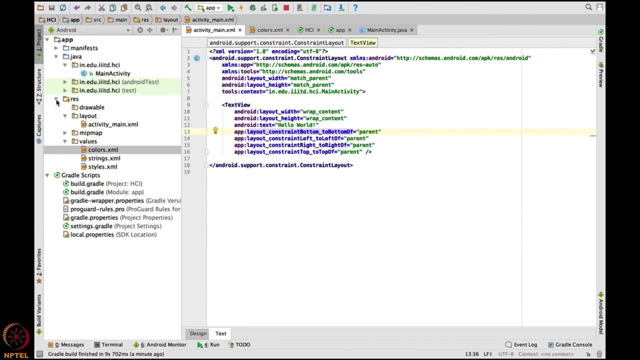 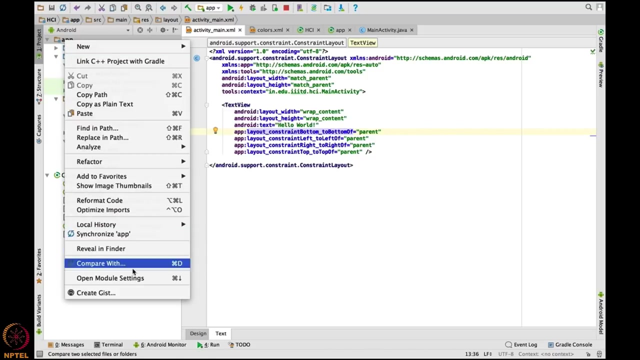 download this. This will download and this will save on your system. You can go back to your app and under the app, you want to create a folder called assets. So basically, font is one of the additional assets of the app, hence the name assets. So what I'm going to do is I'm going to reveal: 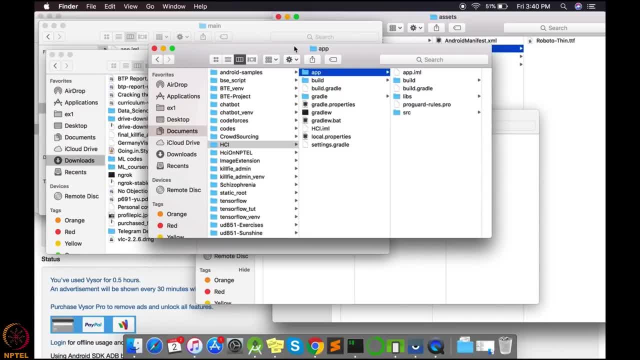 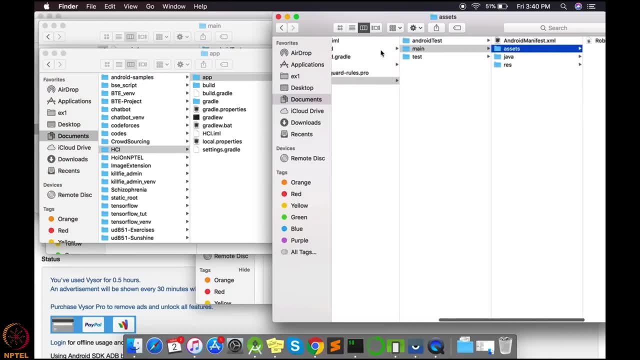 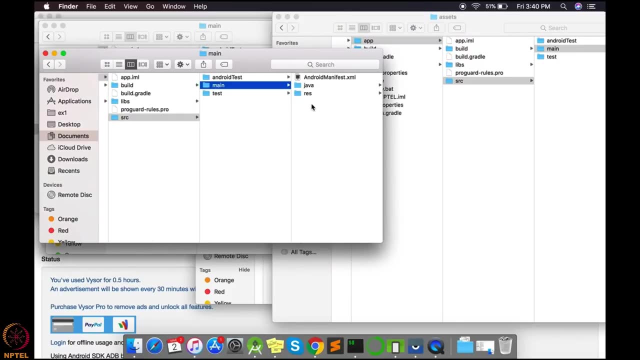 this in finder And this is my app. So this is my app. I'll go in the source, I'll go to main And this place where you can see java and res, I'll create a folder called assets. Now, this is where you should. 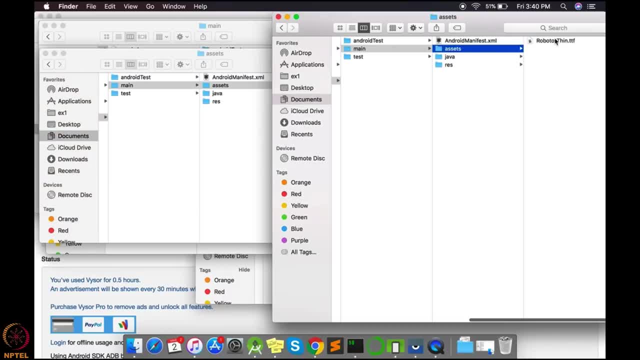 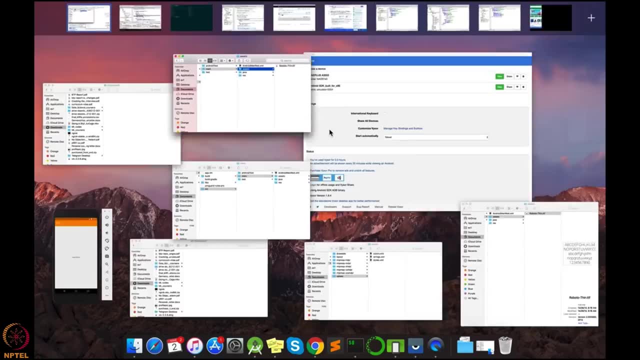 place your font file. So I've already downloaded it: Roboto thin dot tff. dot. tff is basically the extension for all the fonts, So just place it in the assets folder And this should reflect here, so, like you can see, there's an assets folder which is being created with your 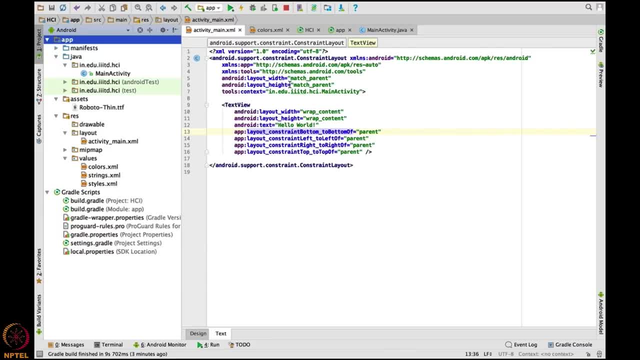 font file. okay, so far, so good. now we want the text to be written in this view. text view is basically the element which renders the text hello world like we saw. so I want the hello world, which was in Roboto earlier, to now be in Roboto thin. 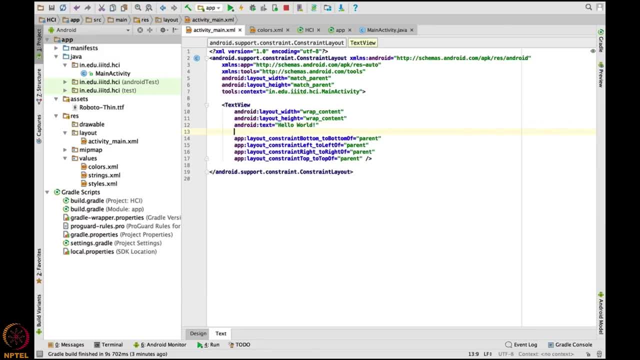 so we'll look at how to do that. first let's just change the text size. so just to make it more legible, I'm setting the text size to be 50 SP now. now I want to change the font to, let's say, Roboto thin. how to do that? so for that we'll have to. 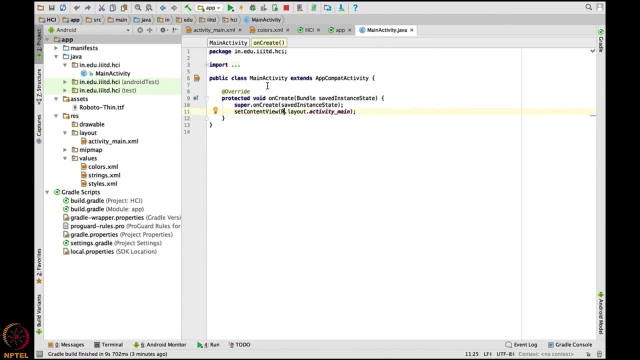 go to our main activity, which is the back end. now, if you do not understand this code, that's fine. this is already. this is pre-rendered code by Google, so you do not need to understand it. all you need to do is this is Java code, so just. 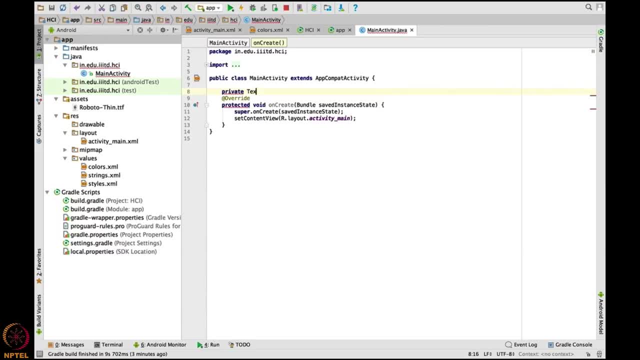 declare a variable which is private text to you and give it any main text to you. so this is the variable name, this is the variable type and you might want to import this and here in on create. so on, create is a callback and this function is called whenever an app is started or 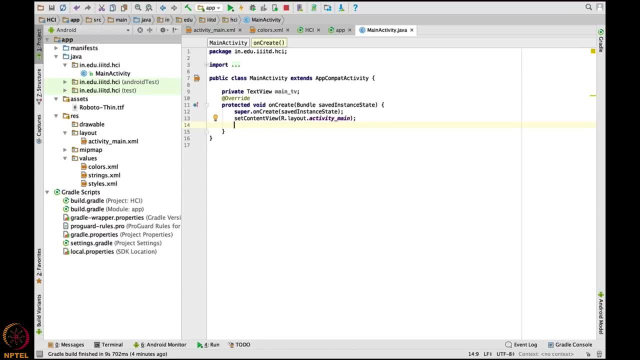 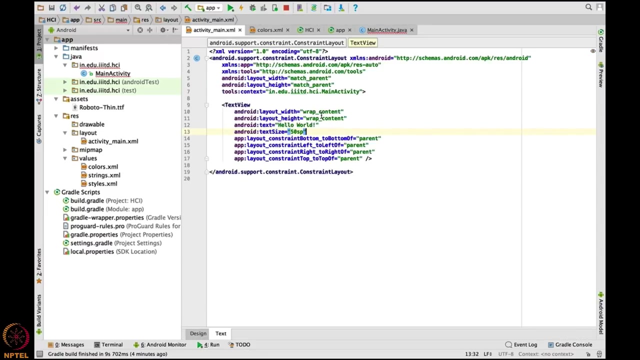 whenever an app is created. and when is an app created? whenever you fire up an app, that's when it creates all the elements. so whatever code is written in this on create function will be executed then. so I'll just quickly show you. so what find view by ID does is. I have declared my view here and I want to 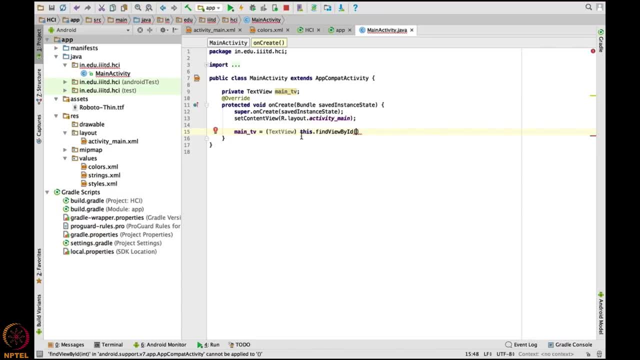 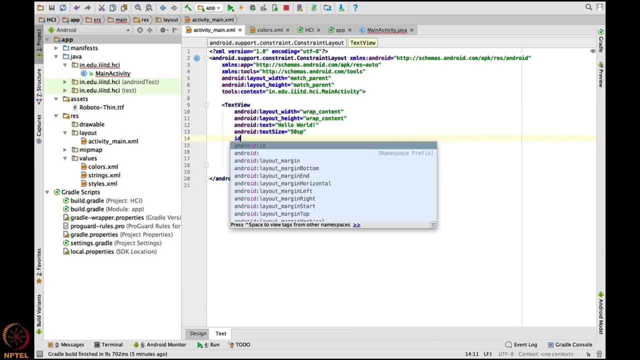 capture that view in my back end. so this is basically just indicating I'm referring to main activity, which is my only activity as of now. this dot find view by ID and our dirt ID dot. so I first need to set the ID as well here. so Android ID, just set whatever ID. 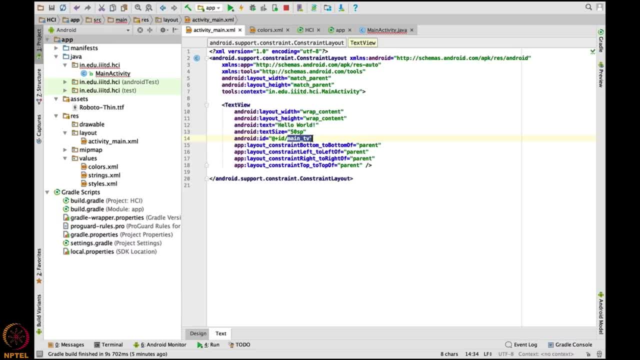 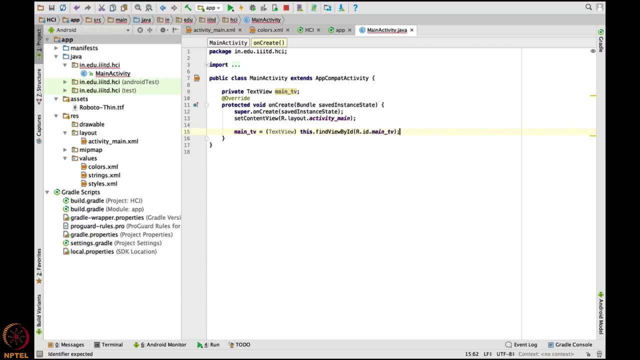 you want to. this can be anything. I just set it as main underscore TV for a main text: you. so here you can be: R dot, ID dot, main TV. so this gets the element in the front end to the back end, and now you can actually set the font here. so you. 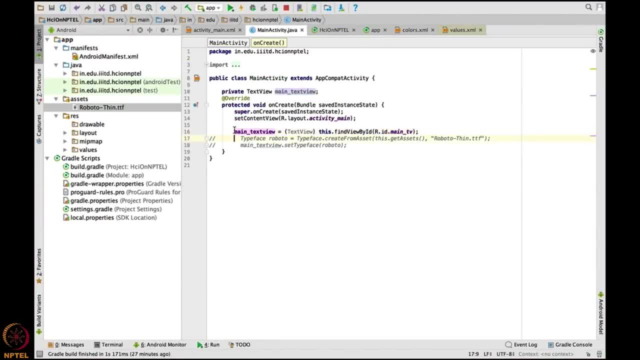 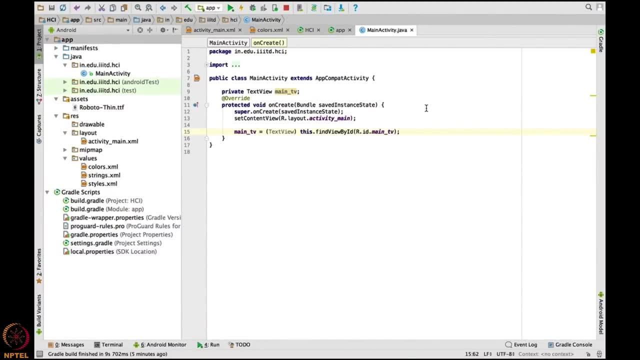 done it. so, yeah, something like this. so so in android studio you cannot set a custom font which you've downloaded from the front end. that's why you need to capture the text view at the back end and do this. so typeface is the is like the name's, just it's it. it defines how a view looks like. what is the font going to be? so 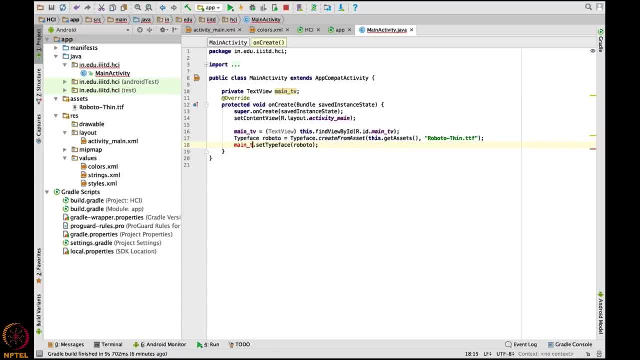 so declare a typeface object i do create from asset. create from asset because i saved it in the assets folder. this dot get assets. this basically gets all the things in the assets folder and roboto thin dot tff, which is the filing. so again, if you do not understand the 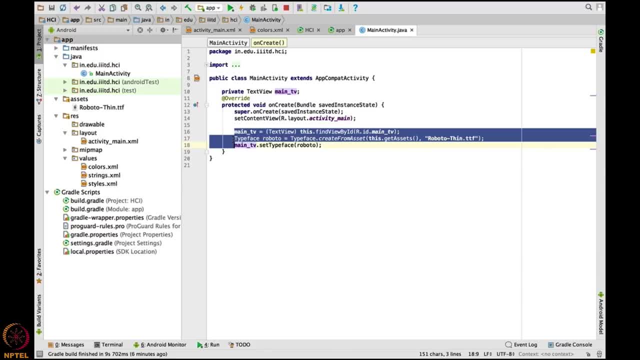 code part of this. that's fine. just copy paste this code. this should work. we're more focused on the design part of things, so i just set the typeface as roboto and this should set you my font in this field to roboto thin. so let's just see if that got implemented.